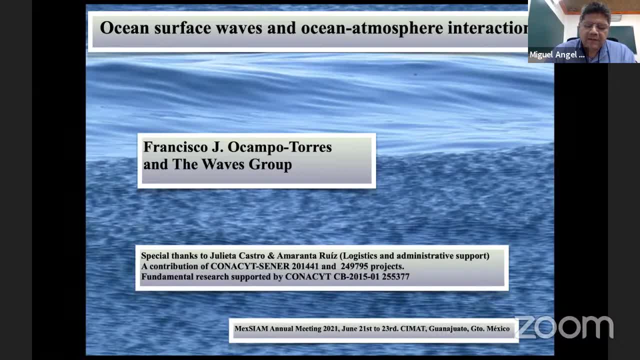 in ocean wave energy and the potential conversion to practical uses. dealing with resources, evaluation and with the development of experiments in the laboratory and at sea To make progress on designing and building new devices to convert the ocean wave energy. Supervisor or co-supervisor. 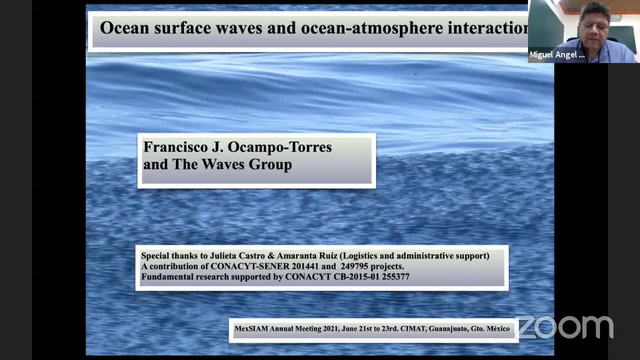 of about 30 graduate students, 11 PhD and 21 Master of Sciences. He's an active member of the Waves in Shell Environments group since 1994, and of his scientific committee since 2014.. Member of the Mexican Academy of Sciences since 2000,- 2000, and of the Mexican National 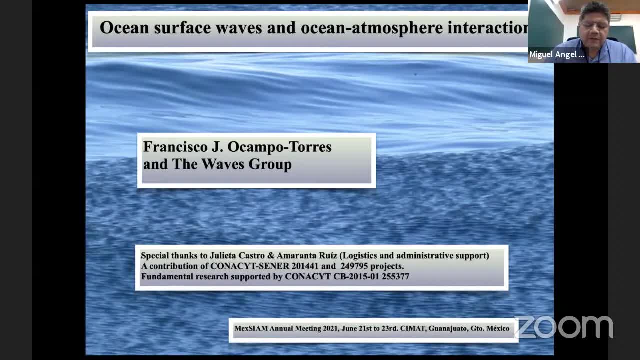 Research Institute. Thank you All right. Good morning everyone. Thanks very much for this introduction and especially for this opportunity that you can provide us in order to have you an idea of what we are doing in the Waves group regarding ocean surface waves and ocean-atmosphere interactions. 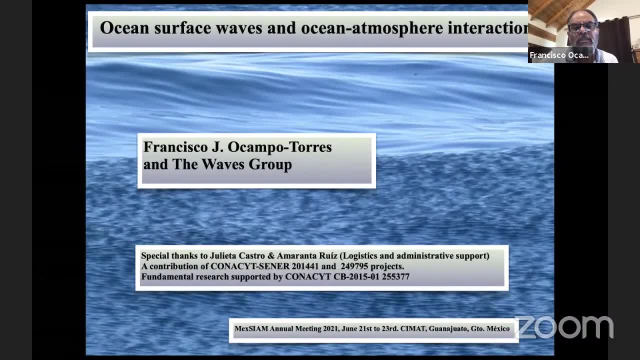 I would like to acknowledge and thanks Julieta Castro and Amaranta Ruiz for their great support, mainly in logistics and administrative procedures. This research has established a very strong relationship with the ocean and the ocean And I would like to acknowledge and thank Julieta Castro and Amaranta Ruiz for their great support, mainly in logistics and administrative. 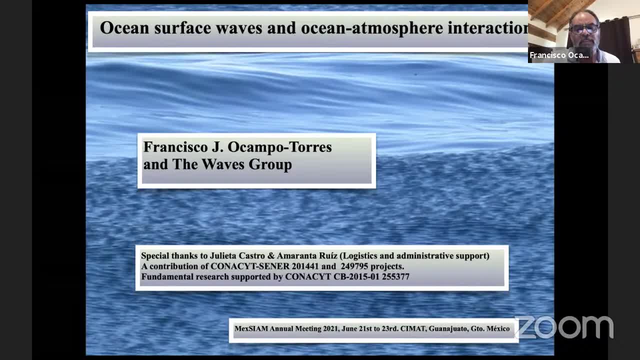 procedures. This research has established a very strong relationship with the ocean and the ocean And I would like to acknowledge and thanks Julieta Castro and Amaranta Ruiz for their great support, mainly in logistics and administrative procedures. This research has established a very strong relationship with the ocean and the ocean And I would like 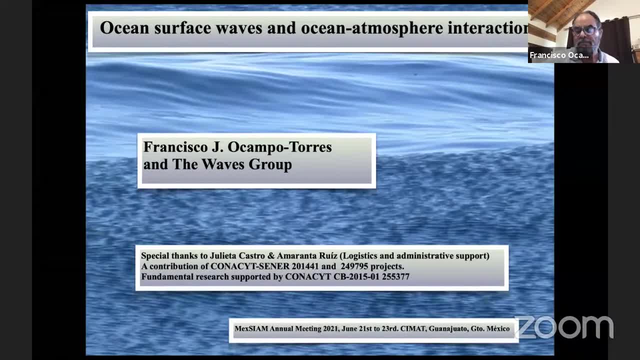 to acknowledge and thanks Julieta Castro and Amaranta Ruiz for their great support, mainly in logistics and administrative procedures. This research has established a very strong relationship with the ocean and the ocean And I would like to acknowledge and thanks Julieta Castro and Amaranta Ruiz for their great support, mainly in logistics and administrative. 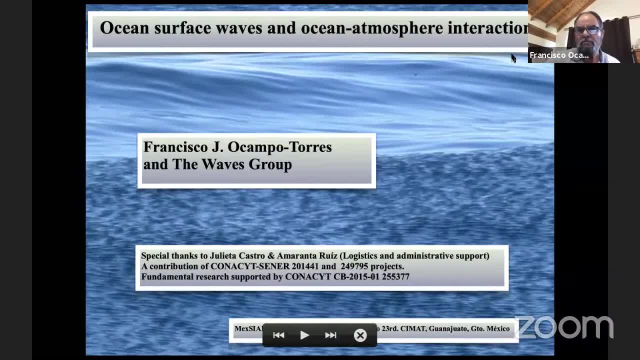 procedures. This research has established a very strong relationship with the ocean and the ocean And I would like to acknowledge and thanks Julieta Castro and Amaranta Ruiz for their great support, mainly in logistics and administrative procedures. This research has established a very strong relationship with the ocean and the ocean And I would like to acknowledge 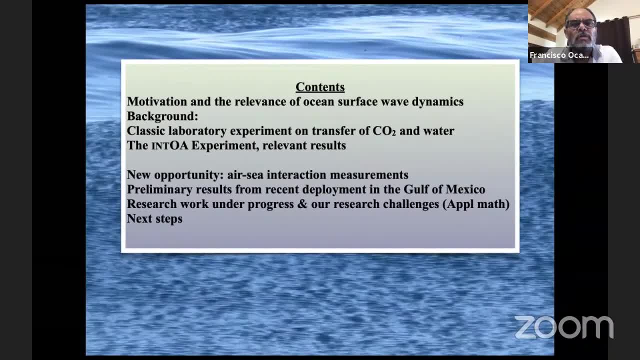 and thanks Julieta Castro and Amaranta Ruiz for their great support, mainly in logistics and administrative procedures. This research has established a very strong relationship with the ocean and the ocean And I would like to acknowledge and thanks Julieta Castro and Amaranta Ruiz for their great support, mainly in logistics and administrative procedures. 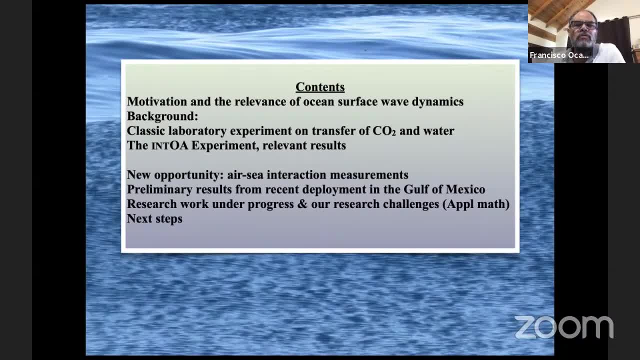 This research has established a very strong relationship with the ocean and the ocean And I would like to acknowledge and thanks Julieta Castro and Amaranta Ruiz for their great support, mainly in logistics and administrative procedures. This research has established a very strong relationship with the ocean and the ocean And I would like to acknowledge 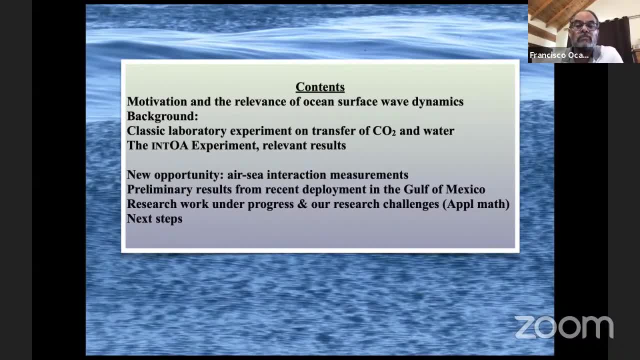 and thanks Julieta Castro and Amaranta Ruiz for their great support, mainly in logistics and administrative procedures. This research has established a very strong relationship with the ocean and the ocean And I would like to acknowledge and thanks Julieta Castro and Amaranta Ruiz for their great support, mainly in logistics and administrative procedures. This research 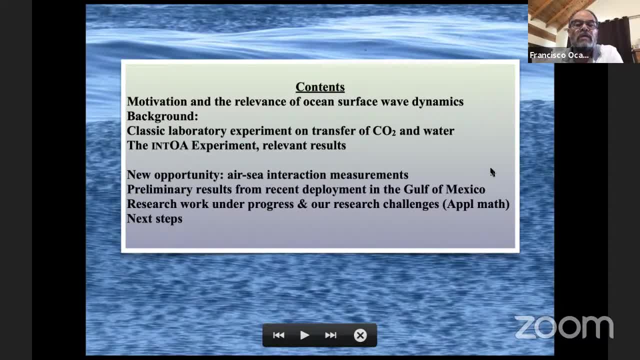 has established a very strong relationship with the ocean and the ocean And I would like to acknowledge and thanks Julieta Castro and Amaranta Ruiz for their great support, mainly in logistics and administrative procedures. This research has established a very strong relationship with the ocean and the ocean And I would like to acknowledge and thanks. 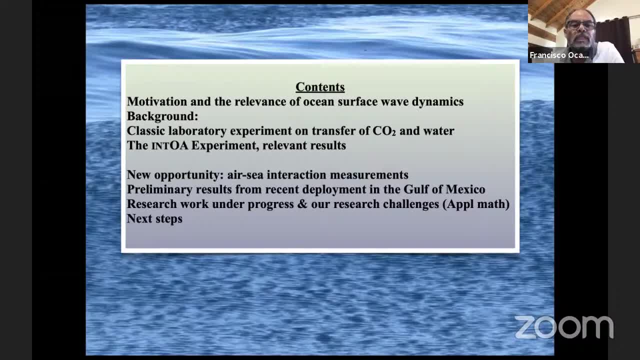 Julieta Castro and Amaranta Ruiz for their great support, mainly in logistics and administrative procedures. This research has established a very strong relationship with the ocean and the ocean And I would like to acknowledge and thanks Julieta Castro and Amaranta Ruiz for their great support, mainly in logistics and administrative procedures. This research 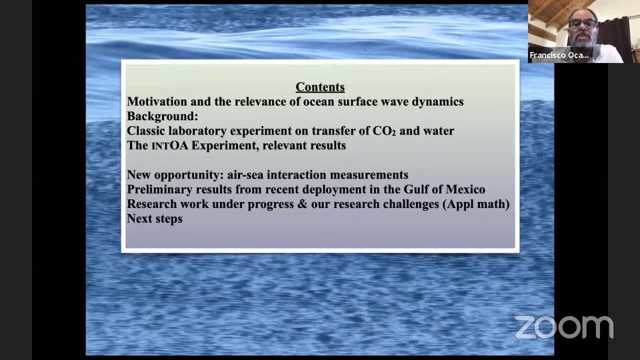 has established a very strong relationship with the ocean and the ocean, And I would like to acknowledge and thanks Julieta Castro and Amaranta Ruiz for their great support, mainly in logistics and administrative procedures. This research has established a very strong relationship with the ocean And I would like to acknowledge and thanks Julieta Castro and Amaranta Ruiz. 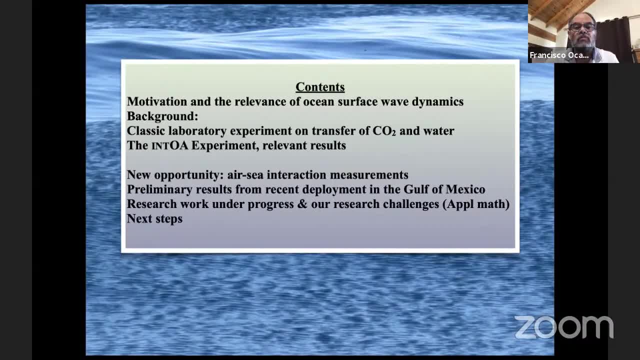 for their great support, mainly in logistics and administrative procedures. This research has established a very strong relationship with the ocean And I would like to acknowledge and thanks Julieta Castro and Amaranta Ruiz for their great support, mainly in logistics and administrative procedures. This research has established a very strong relationship. 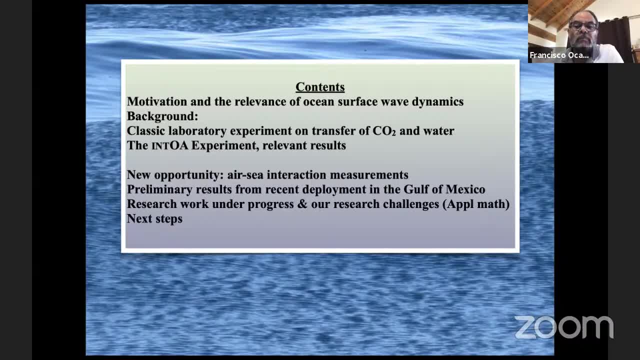 with the ocean And I would like to acknowledge and thanks Julieta Castro and Amaranta Ruiz for their great support, mainly in logistics and administrative procedures. This research has established a very strong relationship with the ocean And I would like to acknowledge and thanks Julieta Castro and Amaranta Ruiz for their great support, mainly in logistics. 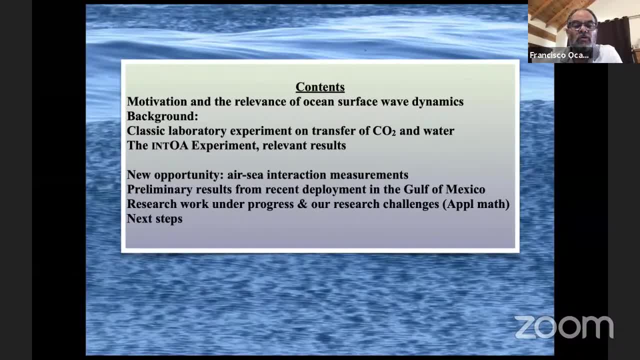 and administrative procedures. This research has established a very strong relationship with the ocean And I would like to acknowledge and thanks Julieta Castro and Amaranta Ruiz for their great support, mainly in logistics and administrative procedures. This research has established a very strong relationship with the ocean And I would like to acknowledge 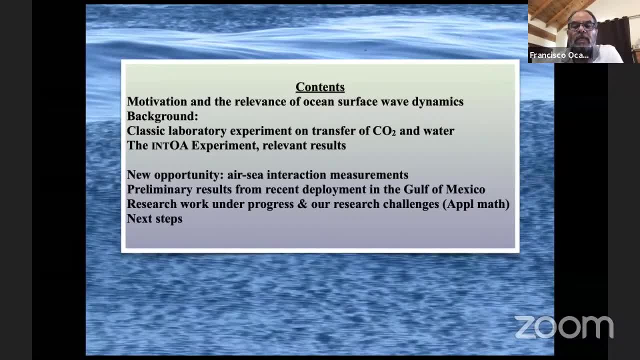 and thanks Julieta Castro and Amaranta Ruiz for their great support, mainly in logistics and administrative procedures. This research has established a very strong relationship with the ocean And I would like to acknowledge and thanks Julieta Castro and Amaranta Ruiz for their great support, mainly in logistics and administrative procedures. This research 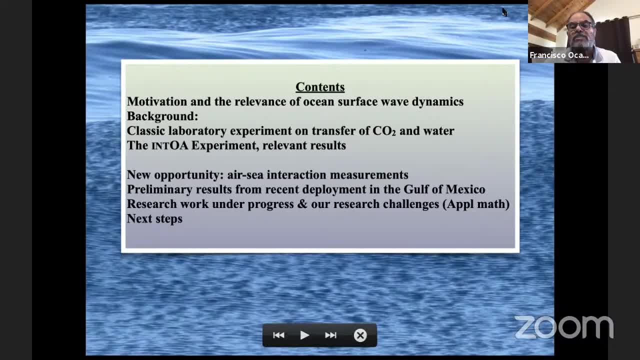 has established a very strong relationship with the ocean And I would like to acknowledge and thanks Julieta Castro and Amaranta Ruiz for their great support, mainly in logistics and administrative procedures. This research has established a very strong relationship with the ocean And I would like to acknowledge and thanks Julieta Castro and Amaranta Ruiz. 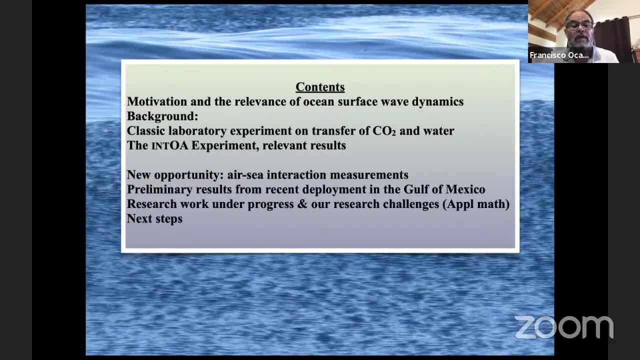 for their great support, mainly in logistics and administrative procedures. This research has established a very strong relationship with the ocean And I would like to acknowledge and thanks Julieta Castro and Amaranta Ruiz for their great support, mainly in logistics and administrative procedures. This research has established a very strong relationship. 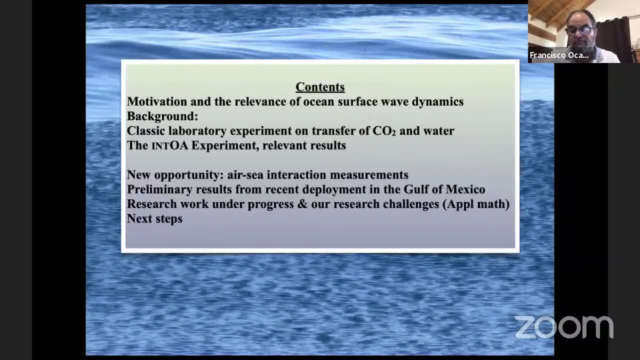 with the ocean And I would like to acknowledge and thanks Julieta Castro and Amaranta Ruiz for their great support, mainly in logistics and administrative procedures. This research has established a very strong relationship with the ocean And I would like to acknowledge and thanks Julieta Castro and Amaranta Ruiz for their great support, mainly in logistics. 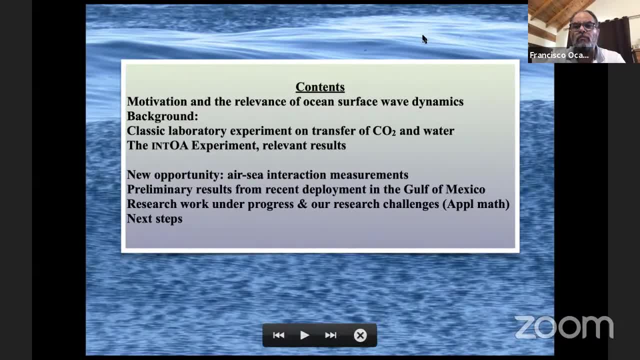 and administrative procedures. This research has established a very strong relationship with the ocean And I would like to acknowledge and thanks Julieta Castro and Amaranta Ruiz for their great support, mainly in logistics and administrative procedures. This research has established a very strong relationship with the ocean And I would like to acknowledge 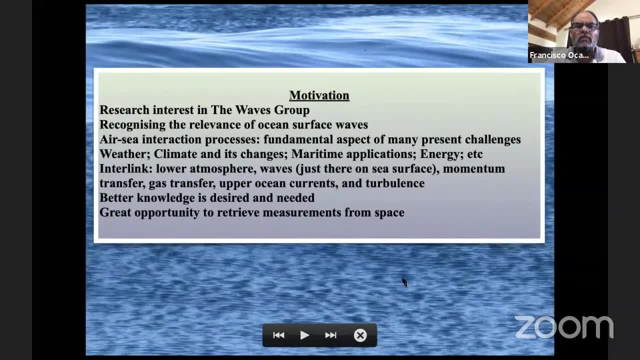 and thanks Julieta Castro and Amaranta Ruiz for their great support, mainly in logistics and administrative procedures. This research has established a very strong relationship with the ocean And I would like to acknowledge and thanks Julieta Castro and Amaranta Ruiz for their great support, mainly in logistics and administrative procedures. This research 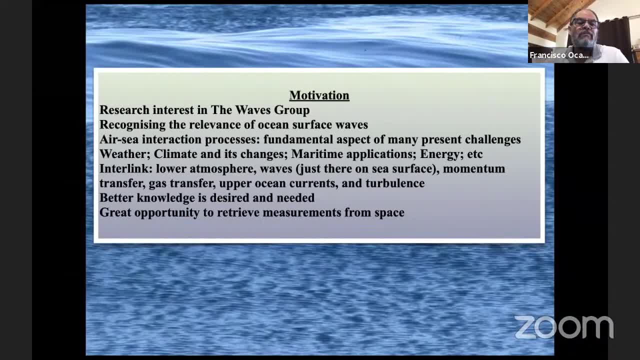 has established a very strong relationship with the ocean And I would like to acknowledge and thanks Julieta Castro and Amaranta Ruiz for their great support, mainly in logistics and administrative procedures. This research has established a very strong relationship with the ocean And I would like to acknowledge and thanks Julieta Castro and Amaranta Ruiz. 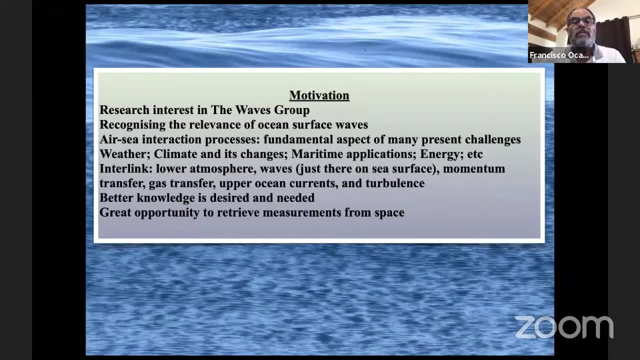 for their great support, mainly in logistics and administrative procedures. This research has established a very strong relationship with the ocean And I would like to acknowledge and thanks Julieta Castro and Amaranta Ruiz for their great support, mainly in logistics and administrative procedures. This research has established a very strong relationship with 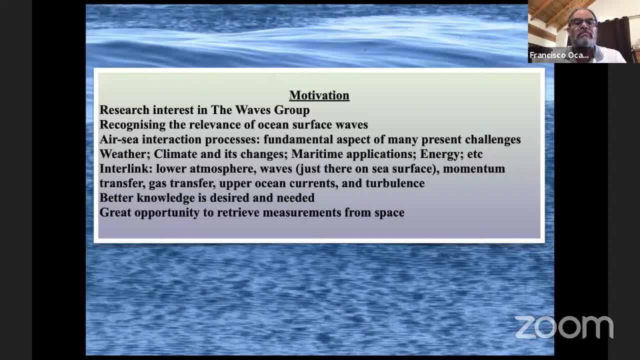 the ocean And I would like to acknowledge and thanks Julieta Castro and Amaranta Ruiz for their great support, mainly in logistics and administrative procedures. This research has established a very strong relationship with the ocean And I would like to acknowledge and thanks Julieta Castro and Amaranta Ruiz for their great support, mainly in logistics. 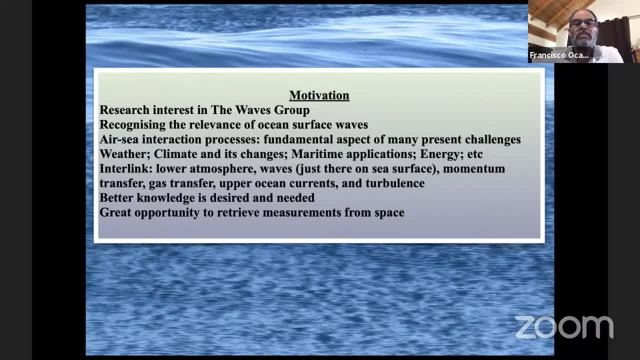 and administrative procedures. This research has established a very strong relationship with the ocean And I would like to acknowledge and thanks Julieta Castro and Amaranta Ruiz for their great support, mainly in logistics and administrative procedures. This research has established a very strong relationship with the ocean And I would like to acknowledge 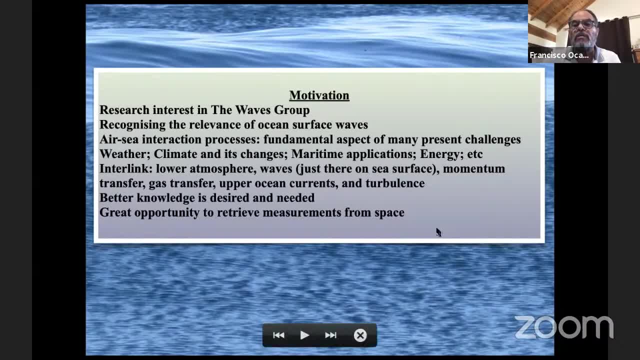 and thanks Julieta Castro and Amaranta Ruiz for their great support, mainly in logistics and administrative procedures. This research has established a very strong relationship with the ocean And I would like to acknowledge and thanks Julieta Castro and Amaranta Ruiz for their great support, mainly in logistics and administrative procedures. This research 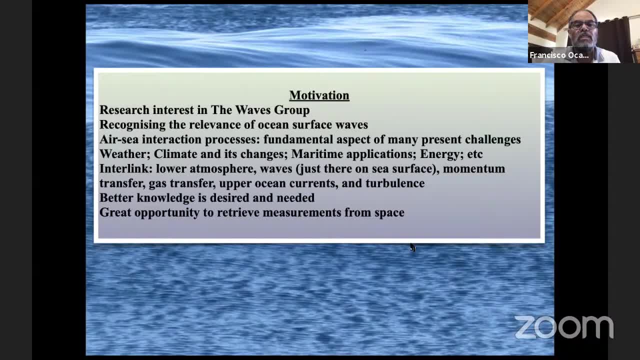 has established a very strong relationship with the ocean And I would like to acknowledge and thanks Julieta Castro and Amaranta Ruiz for their great support, mainly in logistics and administrative procedures. This research has established a very strong relationship with the ocean And I would like to acknowledge and thanks Julieta Castro and Amaranta Ruiz. 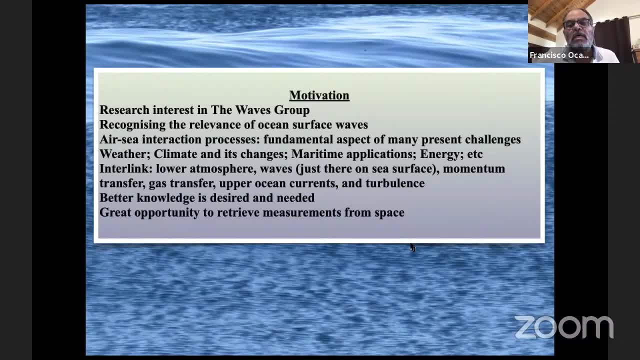 for their great support, mainly in logistics and administrative procedures. This research has established a very strong relationship with the ocean And I would like to acknowledge and thanks Julieta Castro and Amaranta Ruiz for their great support, mainly in logistics and administrative procedures. This research has established a very strong relationship. 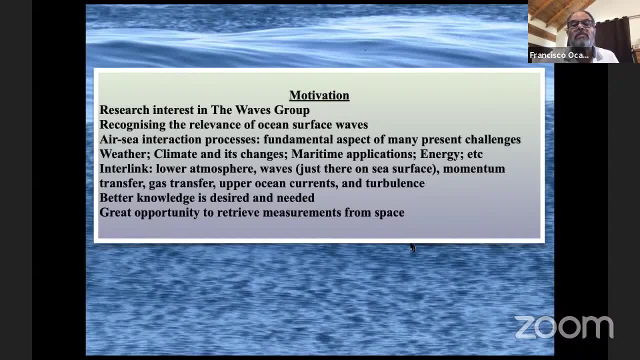 with the ocean And I would like to acknowledge and thanks Julieta Castro and Amaranta Ruiz for their great support, mainly in logistics and administrative procedures. This research has established a very strong relationship with the ocean And I would like to acknowledge and thanks Julieta Castro and Amaranta Ruiz for their great support, mainly in logistics. 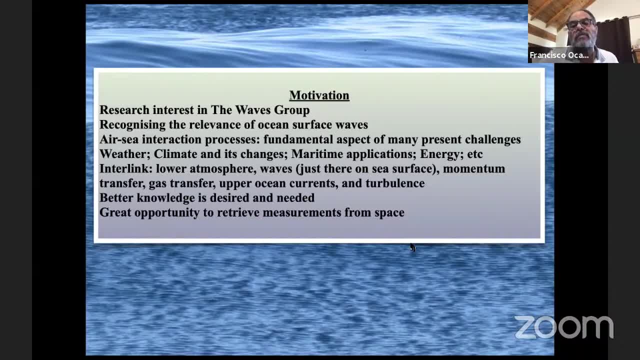 and administrative procedures. This research has established a very strong relationship with the ocean And I would like to acknowledge and thanks Julieta Castro and Amaranta Ruiz for their great support, mainly in logistics and administrative procedures. This research has established a very strong relationship with the ocean And I would like to acknowledge 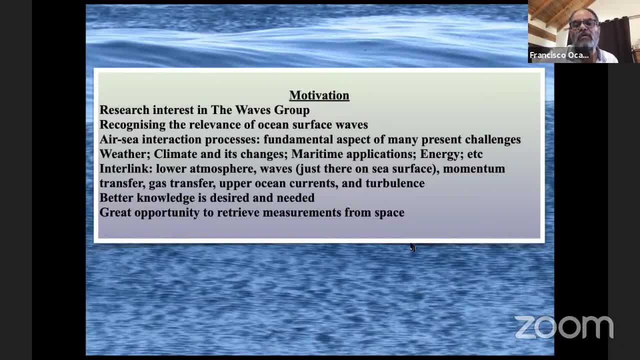 and thanks Julieta Castro and Amaranta Ruiz for their great support, mainly in logistics and administrative procedures. This research has established a very strong relationship with the ocean And I would like to acknowledge and thanks Julieta Castro and Amaranta Ruiz for their great support, mainly in logistics and administrative procedures. This research 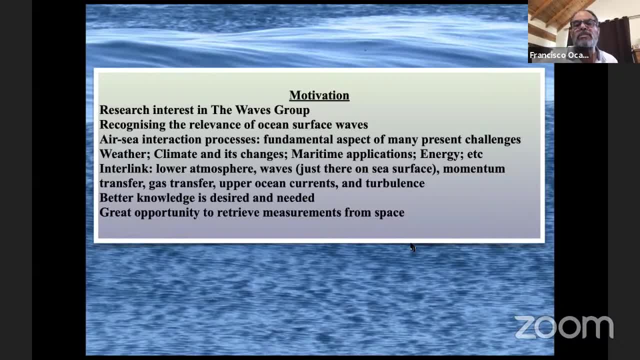 has established a very strong relationship with the ocean And I would like to acknowledge and thanks Julieta Castro and Amaranta Ruiz for their great support, mainly in logistics and administrative procedures. This research has established a very strong relationship with the ocean And I would like to acknowledge and thanks Julieta Castro and Amaranta Ruiz. 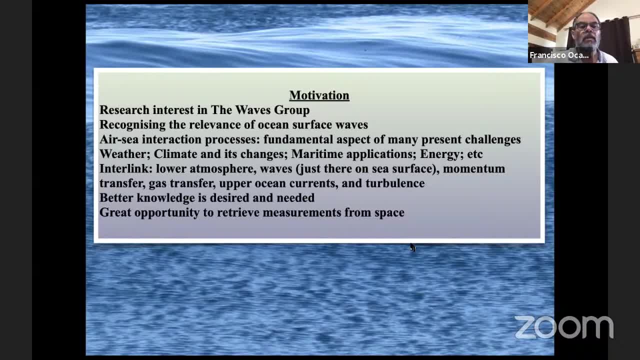 for their great support, mainly in logistics and administrative procedures. This research has established a very strong relationship with the ocean And I would like to acknowledge and thanks Julieta Castro and Amaranta Ruiz for their great support, mainly in logistics and administrative procedures. This research has established a very strong relationship. 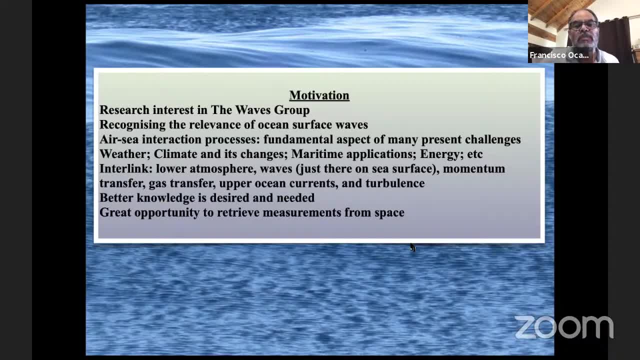 with the ocean And I would like to acknowledge and thanks Julieta Castro and Amaranta Ruiz for their great support, mainly in logistics and administrative procedures. This research has established a very strong relationship with the ocean And I would like to acknowledge and thanks Julieta Castro and Amaranta Ruiz for their great support, mainly in logistics. 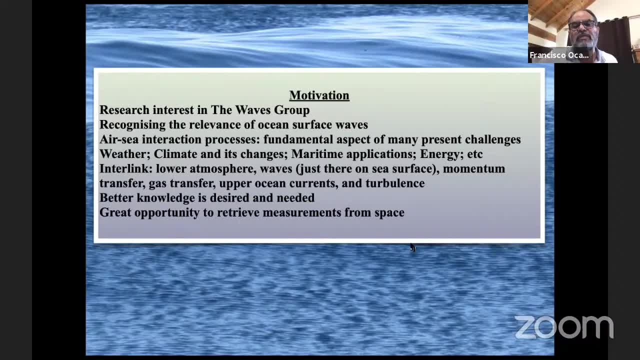 and administrative procedures. This research has established a very strong relationship with the ocean And I would like to acknowledge and thanks Julieta Castro and Amaranta Ruiz for their great support, mainly in logistics and administrative procedures. This research has established a very strong relationship with the ocean And I would like to acknowledge 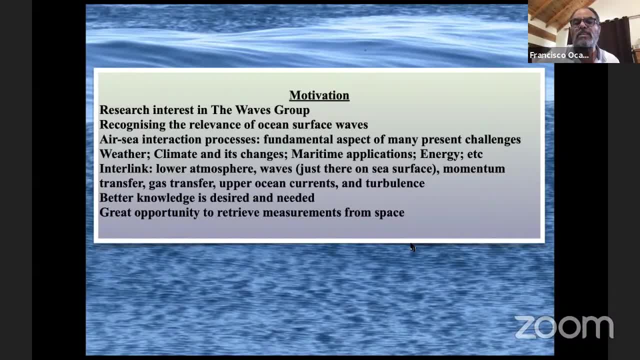 and thanks Julieta Castro and Amaranta Ruiz for their great support, mainly in logistics and administrative procedures. This research has established a very strong relationship with the ocean And I would like to acknowledge and thanks Julieta Castro and Amaranta Ruiz for their great support, mainly in logistics and administrative procedures. This research 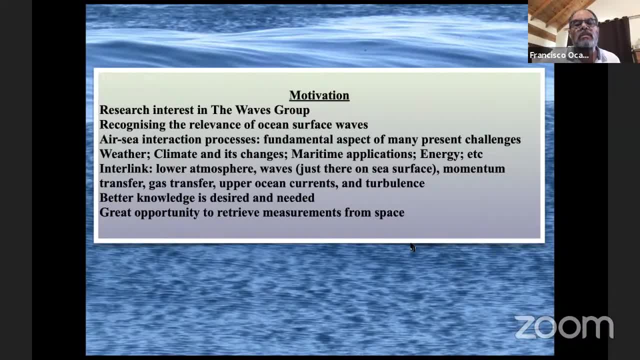 has established a very strong relationship with the ocean And I would like to acknowledge and thanks Julieta Castro and Amaranta Ruiz for their great support, mainly in logistics and administrative procedures. This research has established a very strong relationship with the ocean And I would like to acknowledge and thanks Julieta Castro and Amaranta Ruiz for 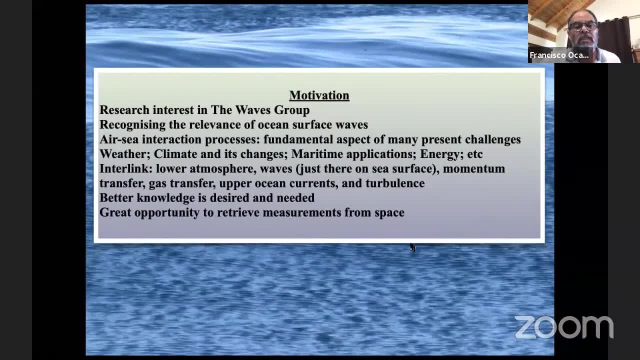 their great support, mainly in logistics and administrative procedures. This research has established a very strong relationship with the ocean And I would like to acknowledge and thanks Julieta Castro and Amaranta Ruiz for their great support, mainly in logistics and administrative procedures. This research has established a very strong relationship. 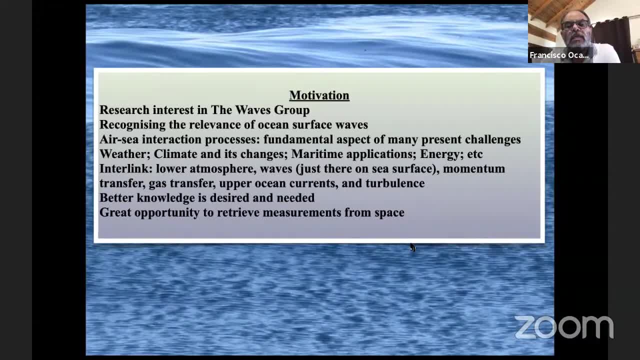 with the ocean And I would like to acknowledge and thanks Julieta Castro and Amaranta Ruiz for their great support, mainly in logistics and administrative procedures. This research has established a very strong relationship with the ocean And I would like to acknowledge and thanks Julieta Castro and Amaranta Ruiz for their great support, mainly in logistics. 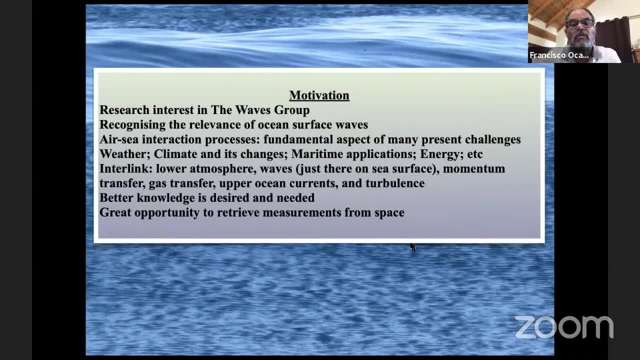 and administrative procedures. This research has established a very strong relationship with the ocean And I would like to acknowledge and thanks Julieta Castro and Amaranta Ruiz for their great support, mainly in logistics and administrative procedures. This research has established a very strong relationship with the ocean And I would like to acknowledge 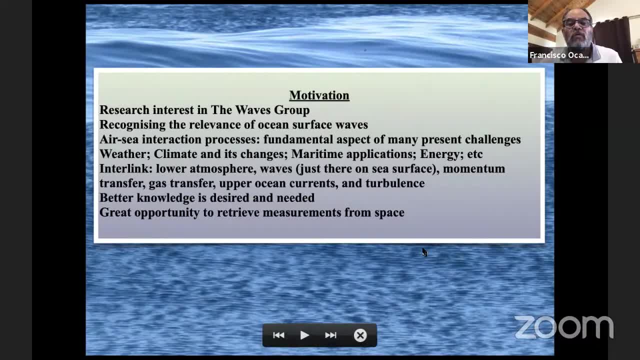 and thanks Julieta Castro and Amaranta Ruiz for their great support, mainly in logistics and administrative procedures. This research has established a very strong relationship with the ocean And I would like to acknowledge and thanks Julieta Castro and Amaranta Ruiz for their great support, mainly in logistics and administrative procedures. This research 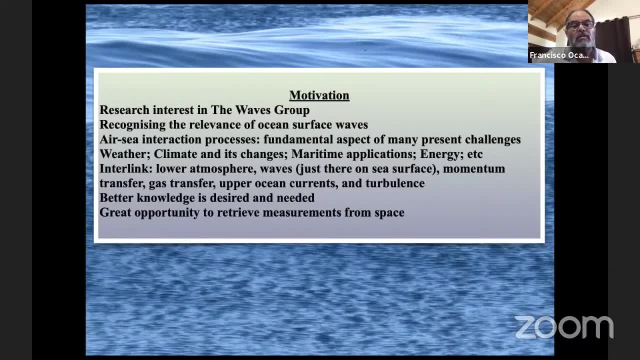 has established a very strong relationship with the ocean And I would like to acknowledge and thanks Julieta Castro and Amaranta Ruiz for their great support, mainly in logistics and administrative procedures. This research has established a very strong relationship with the ocean And I would like to acknowledge and thanks Julieta Castro and Amaranta Ruiz. 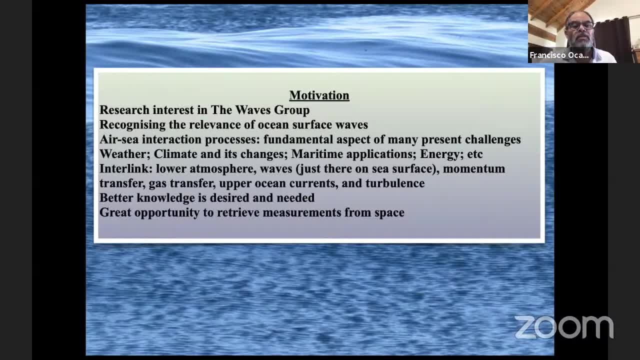 for their great support, mainly in logistics and administrative procedures. This research has established a very strong relationship with the ocean And I would like to acknowledge and thanks Julieta Castro and Amaranta Ruiz for their great support, mainly in logistics and administrative procedures. This research has established a very strong relationship. 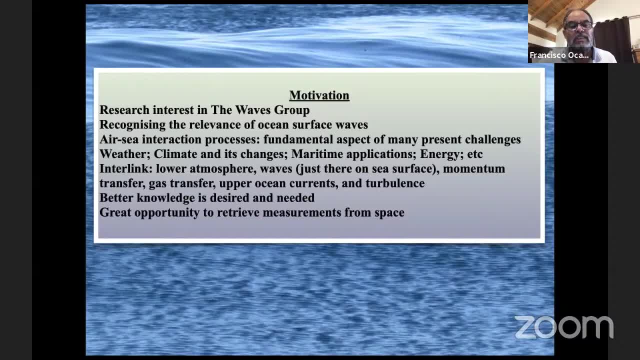 with the ocean And I would like to acknowledge and thanks Julieta Castro and Amaranta Ruiz for their great support, mainly in logistics and administrative procedures. This research has established a very strong relationship with the ocean And I would like to acknowledge and thanks Julieta Castro and Amaranta Ruiz for their great support, mainly in logistics. 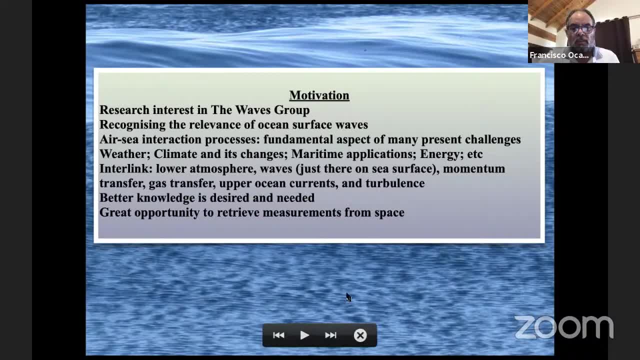 and administrative procedures. This research has established a very strong relationship with the ocean And I would like to acknowledge and thanks Julieta Castro and Amaranta Ruiz for their great support, mainly in logistics and administrative procedures. This research has established a very strong relationship with the ocean And I would like to acknowledge 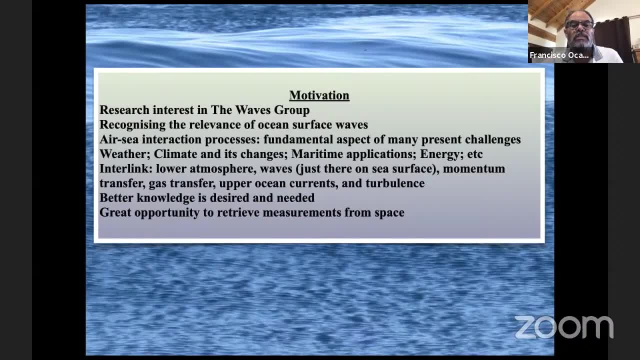 and thanks Julieta Castro and Amaranta Ruiz for their great support, mainly in logistics and administrative procedures. This research has established a very strong relationship with the ocean And I would like to acknowledge and thanks Julieta Castro and Amaranta Ruiz for their great support, mainly in logistics and administrative procedures. This research 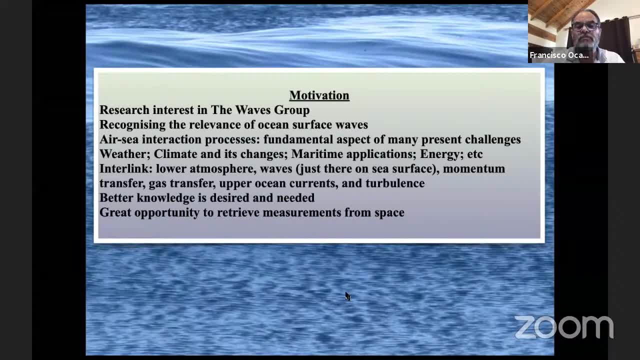 has established a very strong relationship with the ocean And I would like to acknowledge and thanks Julieta Castro and Amaranta Ruiz for their great support, mainly in logistics and administrative procedures. This research has established a very strong relationship with the ocean And I would like to acknowledge and thanks Julieta Castro and Amaranta Ruiz. 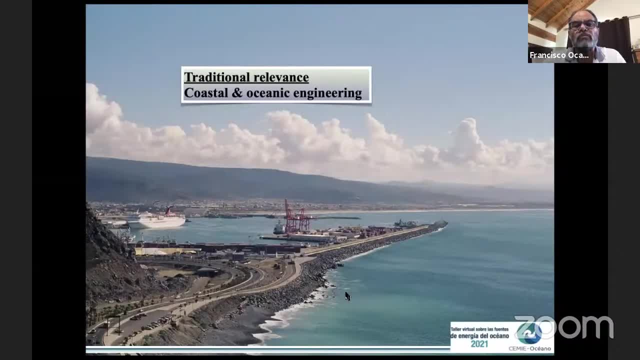 for their great support, mainly in logistics and administrative procedures. This research has established a very strong relationship with the ocean And I would like to acknowledge and thanks Julieta Castro and Amaranta Ruiz for their great support, mainly in logistics and administrative procedures. This research has established a very strong relationship with 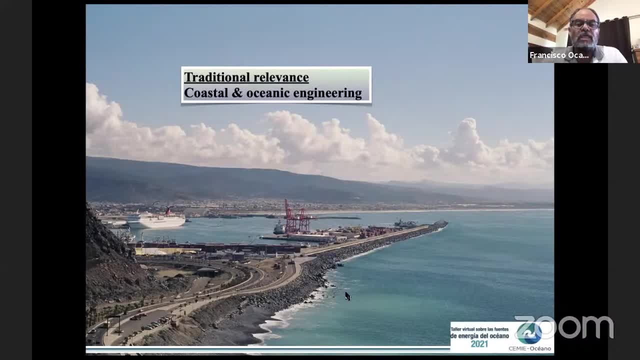 the ocean And I would like to acknowledge and thanks Julieta Castro and Amaranta Ruiz for their great support, mainly in logistics and administrative procedures. This research has established a very strong relationship with the ocean And I would like to acknowledge and thanks Julieta Castro and Amaranta Ruiz for their great support, mainly in logistics. 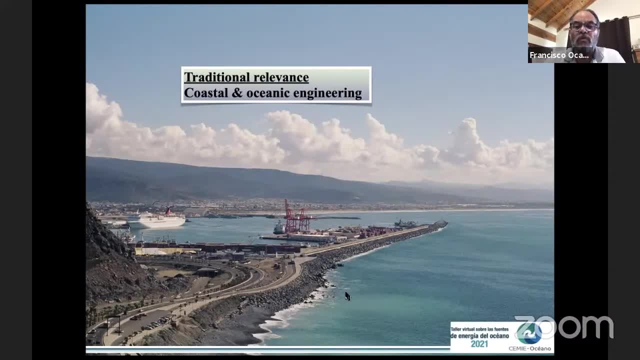 and administrative procedures. This research has established a very strong relationship with the ocean And I would like to acknowledge and thanks Julieta Castro and Amaranta Ruiz for their great support, mainly in logistics and administrative procedures. This research has established a very strong relationship with the ocean And I would like to acknowledge 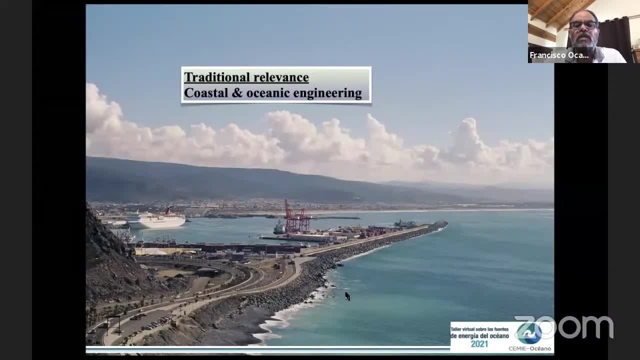 and thanks Julieta Castro and Amaranta Ruiz for their great support, mainly in logistics and administrative procedures. This research has established a very strong relationship with the ocean And I would like to acknowledge and thanks Julieta Castro and Amaranta Ruiz for their great support, mainly in logistics and administrative procedures. This research has 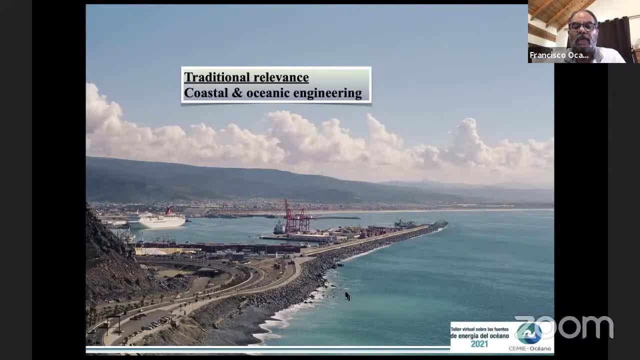 established a very strong relationship with the ocean And I would like to acknowledge and thanks Julieta Castro and Amaranta Ruiz for their great support, mainly in logistics and administrative procedures. This research has established a very strong relationship with the ocean And I would like to acknowledge and thanks Julieta Castro and Amaranta Ruiz. 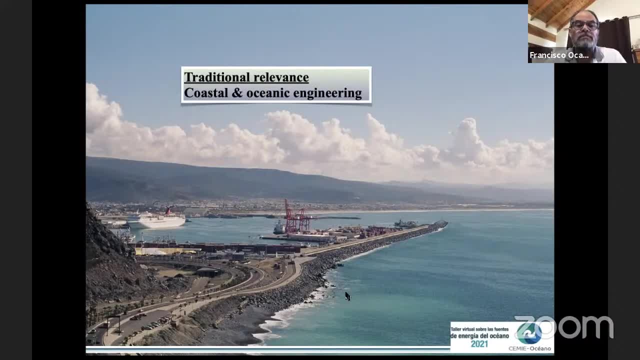 for their great support, mainly in logistics and administrative procedures. This research has established a very strong relationship with the ocean And I would like to acknowledge and thanks Julieta Castro and Amaranta Ruiz for their great support, mainly in logistics and administrative procedures. This research has established a very strong relationship. 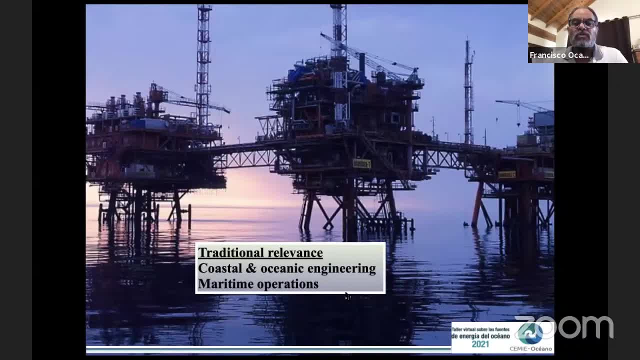 with the ocean And I would like to acknowledge and thanks Julieta Castro and Amaranta Ruiz for their great support, mainly in logistics and administrative procedures. This research has established a very strong relationship with the ocean And I would like to acknowledge and thanks Julieta Castro and Amaranta Ruiz for their great support, mainly in logistics. 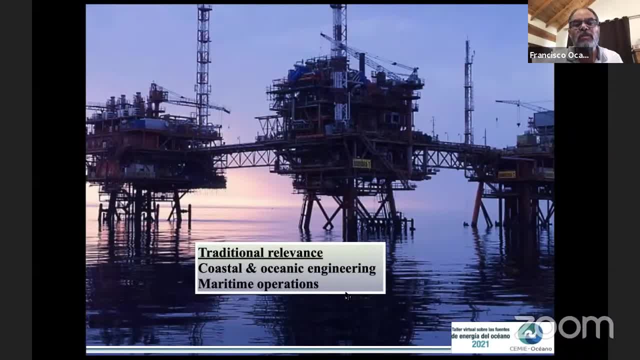 and administrative procedures. This research has established a very strong relationship with the ocean And I would like to acknowledge and thanks Julieta Castro and Amaranta Ruiz for their great support, mainly in logistics and administrative procedures. This research has established a very strong relationship with the ocean And I would like to acknowledge 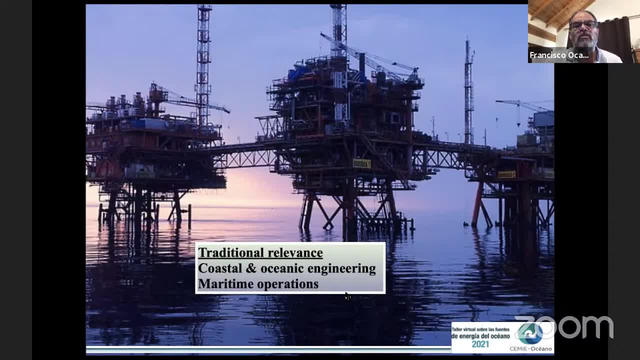 and thanks Julieta Castro and Amaranta Ruiz for their great support, mainly in logistics and administrative procedures. This research has established a very strong relationship with the ocean And I would like to acknowledge and thanks Julieta Castro and Amaranta Ruiz for their great support, mainly in logistics and administrative procedures. This research 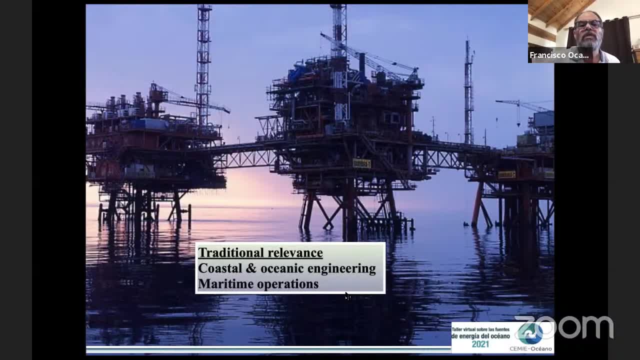 has established a very strong relationship with the ocean And I would like to acknowledge and thanks Julieta Castro and Amaranta Ruiz for their great support, mainly in logistics and administrative procedures. This research has established a very strong relationship with the ocean And I would like to acknowledge and thanks Julieta Castro and Amaranta Ruiz for 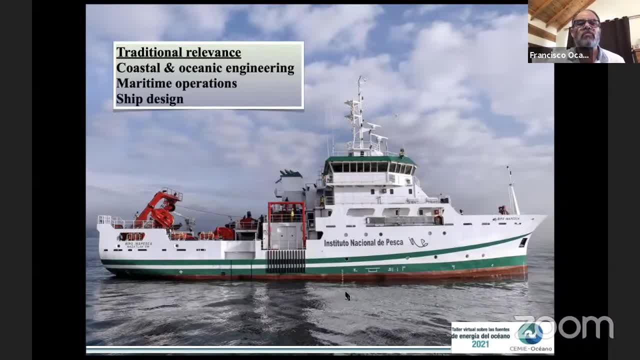 their great support, mainly in logistics and administrative procedures. This research has established a very strong relationship with the ocean And I would like to acknowledge and thanks Julieta Castro and Amaranta Ruiz for their great support, mainly in logistics and administrative procedures. This research has established a very strong relationship. 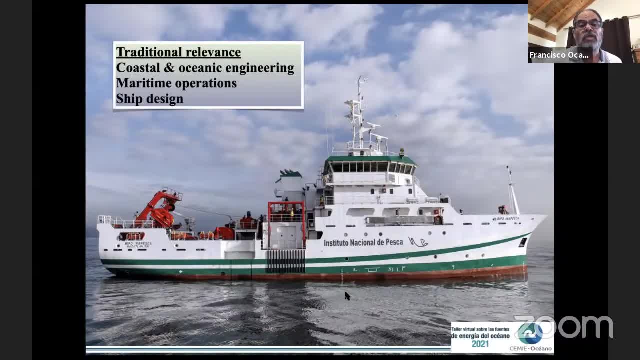 with the ocean And I would like to acknowledge and thanks Julieta Castro and Amaranta Ruiz for their great support, mainly in logistics and administrative procedures. This research has established a very strong relationship with the ocean And I would like to acknowledge and thanks Julieta Castro and Amaranta Ruiz for their great support, mainly in logistics. 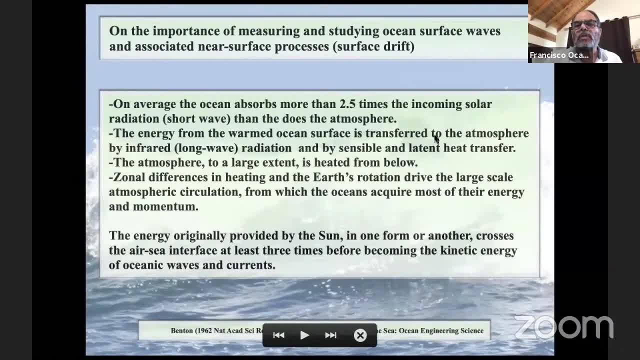 and administrative procedures. This research has established a very strong relationship with the ocean And I would like to acknowledge and thanks Julieta Castro and Amaranta Ruiz for their great support, mainly in logistics and administrative procedures. This research has established a very strong relationship with the ocean And I would like to acknowledge 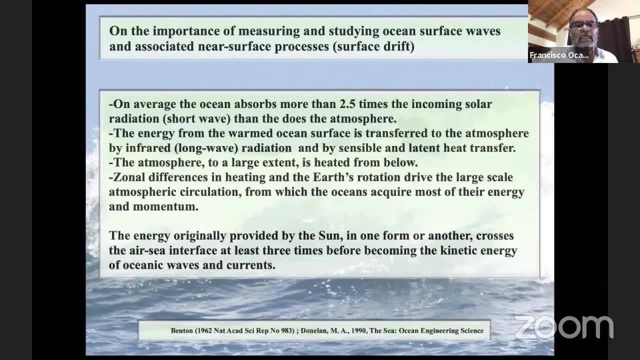 and thanks Julieta Castro and Amaranta Ruiz for their great support, mainly in logistics and administrative procedures. This research has established a very strong relationship with the ocean And I would like to acknowledge and thanks Julieta Castro and Amaranta Ruiz for their great support, mainly in logistics and administrative procedures. This research 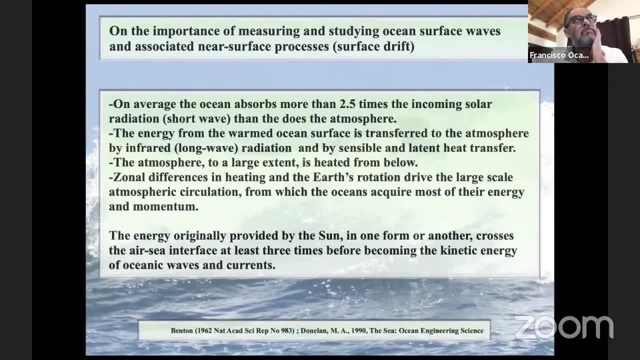 has established a very strong relationship with the ocean And I would like to acknowledge and thanks Julieta Castro and Amaranta Ruiz for their great support, mainly in logistics and administrative procedures. This research has established a very strong relationship with the ocean And I would like to acknowledge and thanks Julieta Castro and Amaranta Ruiz. 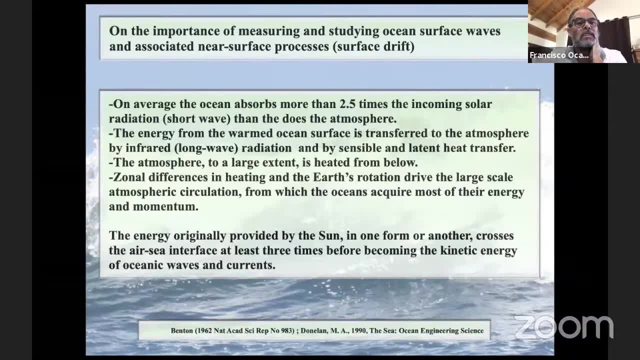 for their great support, mainly in logistics and administrative procedures. This research has established a very strong relationship with the ocean And I would like to acknowledge and thanks Julieta Castro and Amaranta Ruiz for their great support, mainly in logistics and administrative procedures. This research has established a very strong relationship. 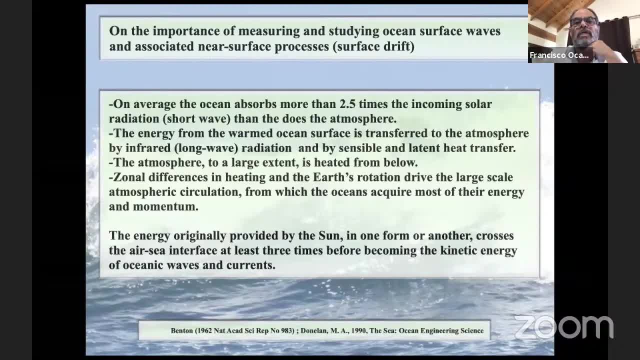 with the ocean And I would like to acknowledge and thanks Julieta Castro and Amaranta Ruiz for their great support, mainly in logistics and administrative procedures. This research has established a very strong relationship with the ocean And I would like to acknowledge and thanks Julieta Castro and Amaranta Ruiz for their great support, mainly in logistics. 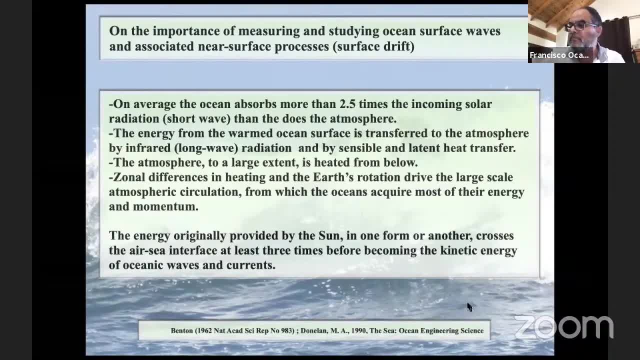 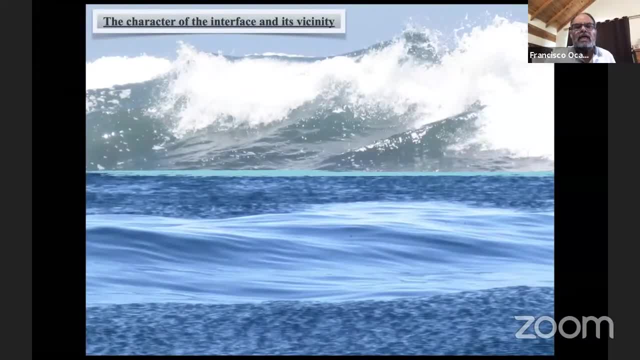 and administrative procedures. This research has established a very strong relationship with the ocean And I would like to acknowledge and thanks Julieta Castro and Amaranta Ruiz for their great support, mainly in logistics, The ocean surface waves And these transfer that we are talking about, of course, going. 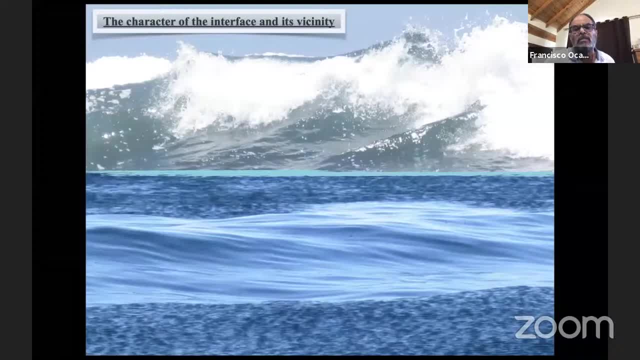 to be very different if we consider the sea surface as a smooth surface or very gently rough, compared to a very high wave surface with current breaking. So we have… We better know the character of the ocean surface waves in order to understand and clearly study the conditions. Thank Julieta Castro and Amaranta Ruiz for their great support, mainly in logistics and administrative procedures. This research has established a very strong connection with the ocean And I would like to acknowledge, And I would like to acknowledge, And I would like to emphasize. and thanks Julieta Castro and Amaranta Ruiz for their great support, mainly in logistics ه. Our research has established a very strong relationship with the ocean And I would like to acknowledge So. we have. we hasn't- we don't know- much information, Robert, so as a to mark, this awakened the vision of a nuevo perforateur. 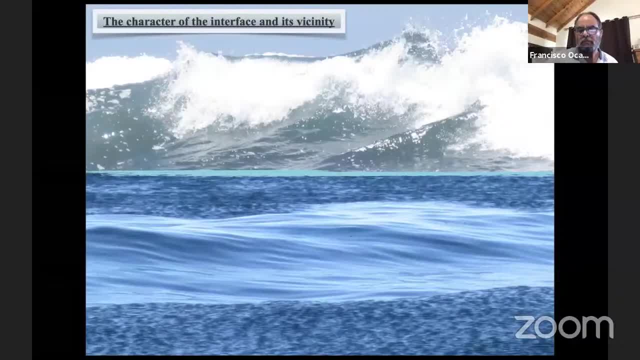 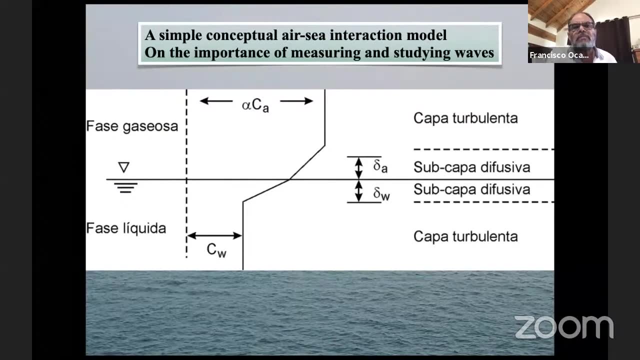 the transfer between the ocean and the atmosphere, for instance in in the case of gases, a very simple, simple conceptual air-sea interaction model is given. in this transparence, we can say that the concentration for any gas above this, above the sea surface, away from the sea surface, can be considered as constant. 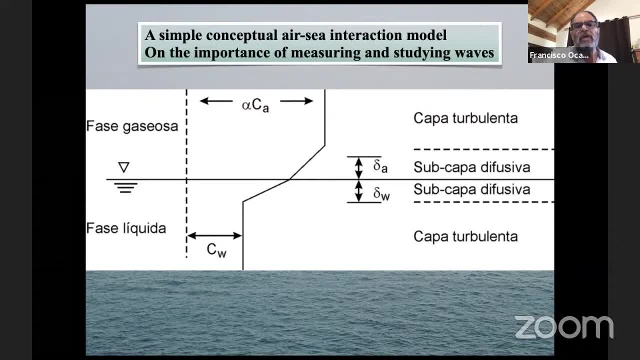 in the vertical and also below the sea surface. away from the sea surface is also constant by different concentrations. but near the sea surface, near the surface interface, there is a sharp increase, sharp gradient of the concentration, because there is a tendency to to be in equilibrium. the the 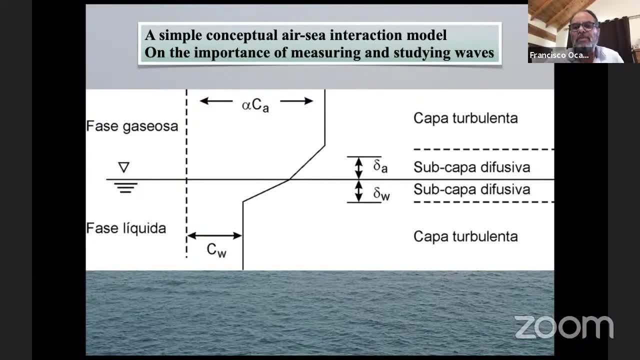 gas above and below. so there is a very thin sub layer, diffusive sub layer, with very sharp gradient in concentration and it is with very sharp gradient in concentration and it is with very sharp gradient in concentration and it is with in these diffusive layers where the 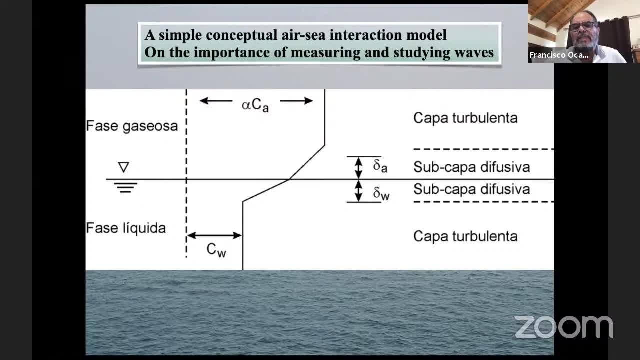 in these diffusive layers where the in these diffusive layers where the resistance to transfer of any property, resistance to transfer of any property, resistance to transfer of any property relies, so you can. you can only think relies, so you can. you can only think relies, so you can. you can only think that any process that disturbs these 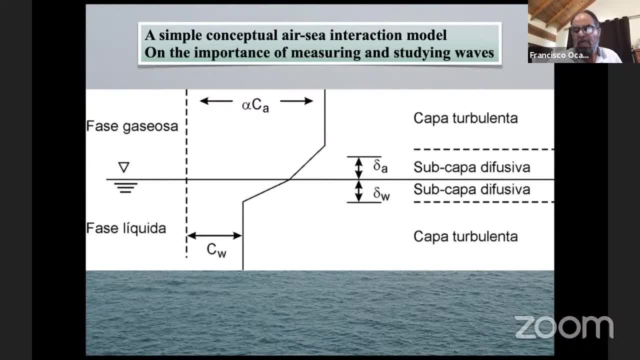 that any process that disturbs these, that any process that disturbs these diffusives of layer could modify or diffusives of layer could modify, or diffusives of layer could modify or modulate the transfer at the whole and modulate the transfer at the whole. and 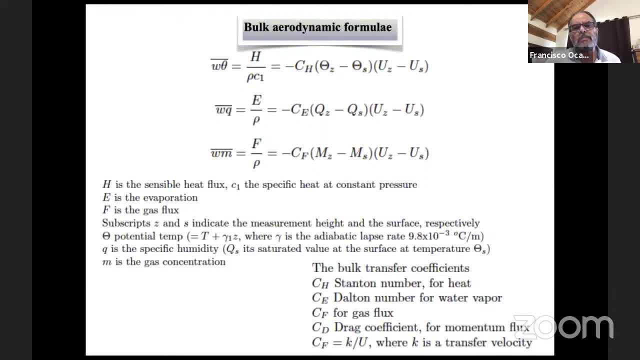 modulate the transfer at the whole and, for instance, in many, for instance in many, for instance in many numerical models, climate models or numerical models, climate models or numerical models, climate models or circulation models. they really rely on circulation models. they really rely on circulation models. they really rely on on book, aerodynamic formula and this. 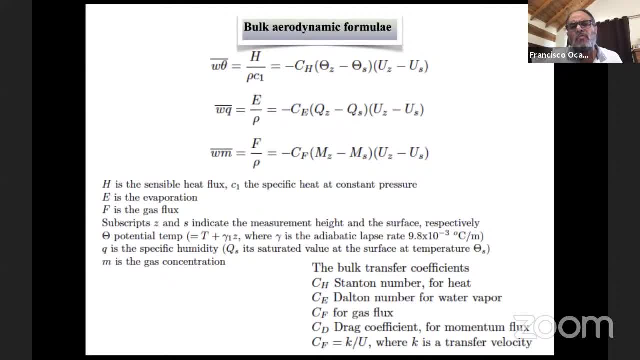 on book aerodynamic formula and this on book aerodynamic formula. and this book aerodynamic formula is a rather book aerodynamic formula is a rather book aerodynamic formula is a rather crude approximation of the flux. in this crude approximation of the flux, in this crude approximation of the flux, in this case we have H, the heat flux, e for the 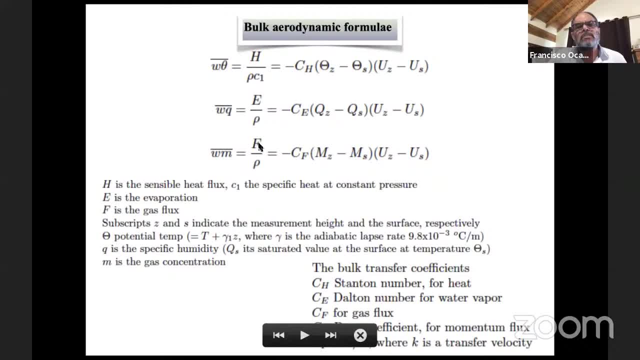 case we have H the heat flux, e for the case we have H the heat flux, e for the evaporation and F for a gas flux. so evaporation and F for a gas flux. so evaporation and F for a gas flux. so they, the models, rely on this. 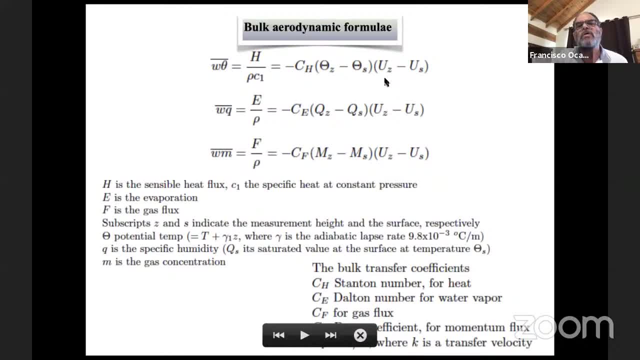 they, the models rely on this. they, the models rely on this. expression on the right where you can, expression on the right where you can, expression on the right, where you can use rather simple variables like mean use, rather simple variables like mean use, rather simple variables like mean wind speed and temperature potential. 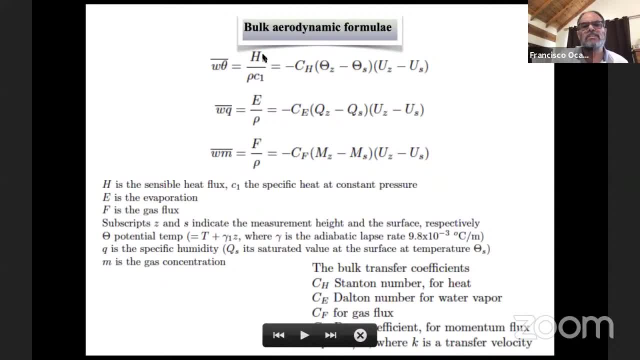 wind speed and temperature, potential wind speed and temperature, potential temperature and so on, to estimate the temperature and so on. to estimate the temperature and so on, to estimate the flux, but in the in a proper way, the flux, but in the in a proper way, the flux, but in the in a proper way the flux can be determined directly if we 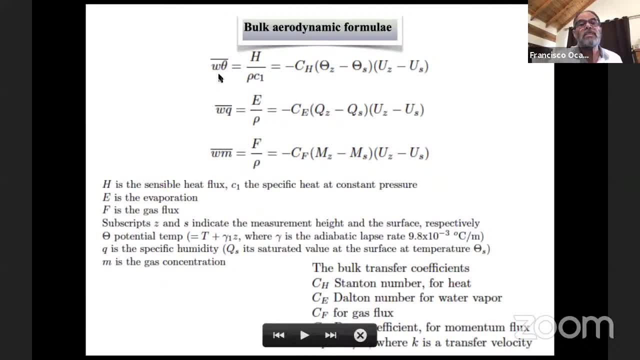 flux can be determined directly. if we flux can be determined directly, if we consider the vertical turbulent of the, consider the vertical turbulent of the, consider the vertical turbulent of the wind component and also the vertical wind component and also the vertical wind component and also the vertical- sorry, the. 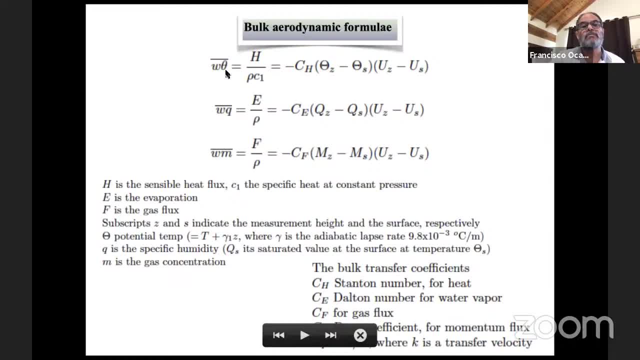 sorry, the a turbulent component of the temperature for the case of heat. Or we can also define the evaporation if we consider the vertical turbulent component of the wind and turbulent component of humidity. And also we can express the flux of a gas if we consider the turbulent component of wind. 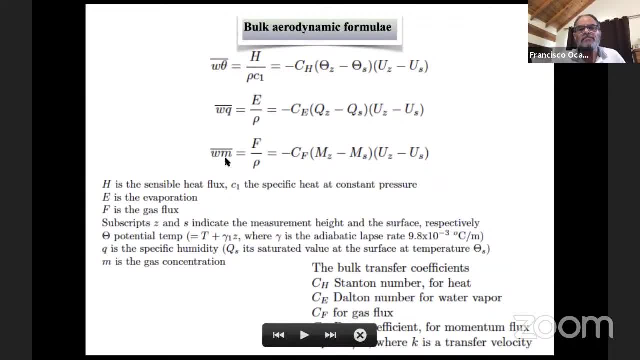 and concentration of that gas. But in the models it is rather difficult to deal with a turbulent variable. So what they do is to rely on this Boolean formula, and rely essentially on these coefficients, which are equivalent to a exchange coefficient of the property that we are dealing with. 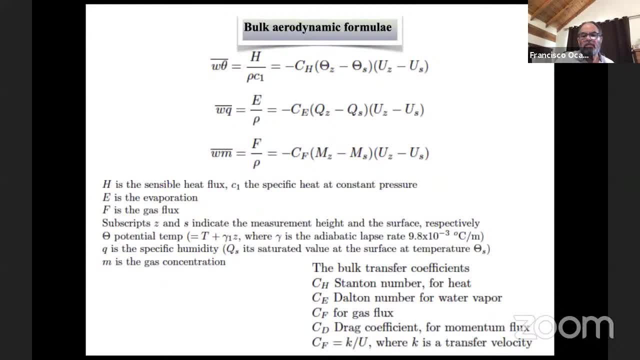 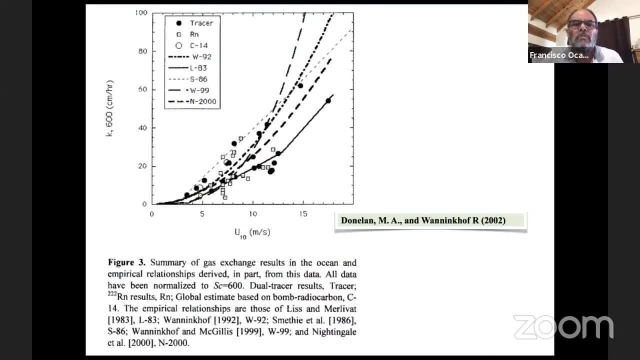 And this exchange coefficient can also be described in terms of the transfer velocity, which is K in this lower part. So this is an example of what transfer velocity of carbon. carbon-bioxide is described as a function of wind speed, U10.. And you can see in these results from Donnelan and Gruaminkoff. 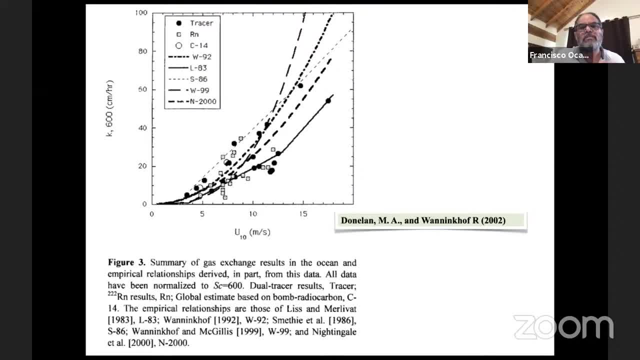 that, depending on the experiment, depending on the data set set, depending on the theoretical analysis, you could. you could deal with either 10 centimeters per hour as transfer velocity, up to 40 when considering, for instance, a mean wind speed of 10 meters per second. so you can, you can see now that if the model, depending on what the model, 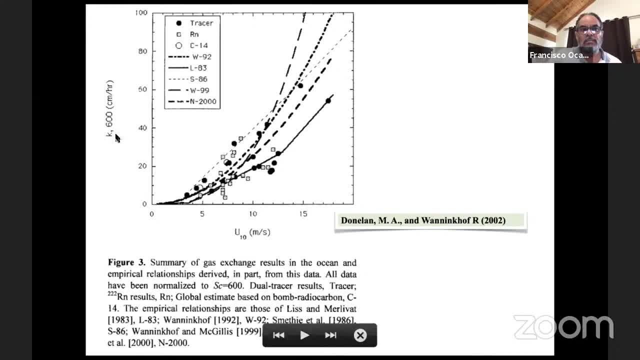 considers as the transfer velocity of co2 as a function of wind speed. even for a case of specific 10 meters per second wind speed, the model will be choosing between 10 or nearly 40 centimeters per hour. so at the end of iterations and time, the the climate that is predicting this. 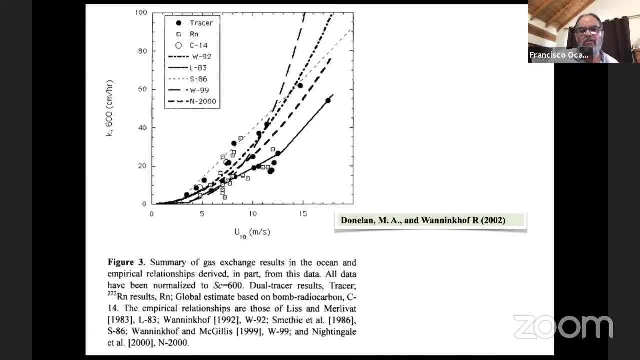 model will be very different depending on what k or transfer velocity is considering. so that's why it's really important to understand better the transfer between c between air and c of co2 and essentially to look at these transfer velocities when not only wind speed is dealing with, but also ocean surface waves. 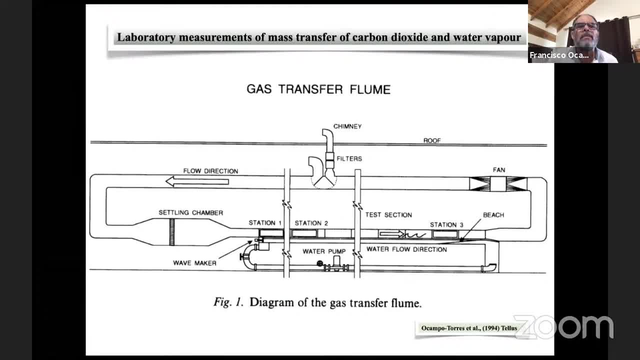 so to get this a little bit, a little bit more clear, i'm gonna show you some classic or historical results that we obtained in a so-called gas transfer film, where we have wind imposed by by a fan on the upper upper tunnel and we have waves in this water tank. 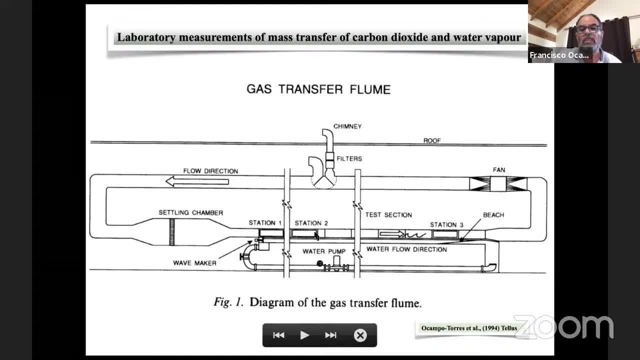 so we measure the waves and at station one, two and three, and we also measure the co2 in the station two of uh simultaneously within the water and within the air. so we run a series of experimental uh tests and for each particular particular wind speed we inject co2 in the water. we close the flaps to make the system closely tightly closed and 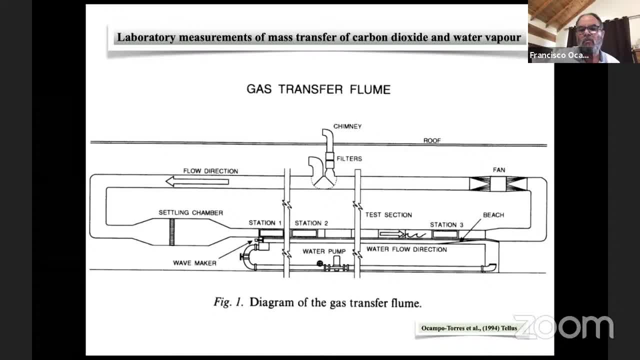 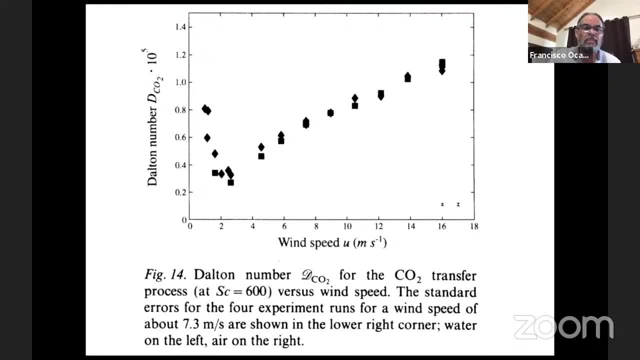 did the measurements to obtain at each experiment one value for the exchange. so the results, as a summary, is this plot for the carbon dioxide uh delta number as a function of wind speed and we can see clearly that the exchange coefficient delta number for co2 decreases with the wind. increases uh from one meter per second. 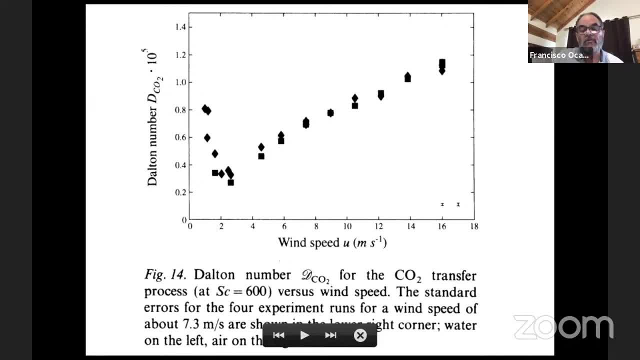 up to three meters per second and for higher wind speeds the exchange coefficient increases slightly, not linearly, but with the wind speed. the results for each symbol is for one particular experiment. so we did many experiments covering wind speed range from 1 to 16 meters per second. we also obtain results for evaporation. so this is the 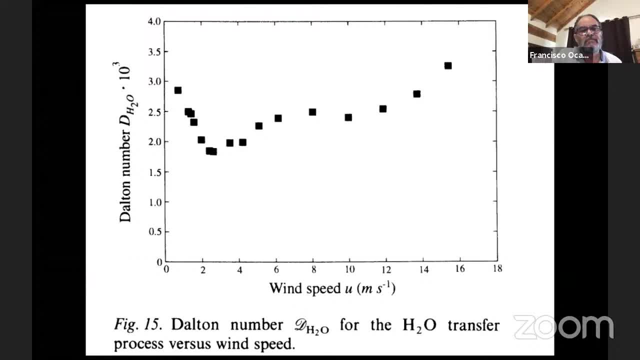 delta number for water, and we can also observe that the exchange coefficient decreases with wind speed, from one meter per second to three meters per second. also the exchange coefficient increases. but we far as being in graduate, so we're going to present this experiment to two子 investing at 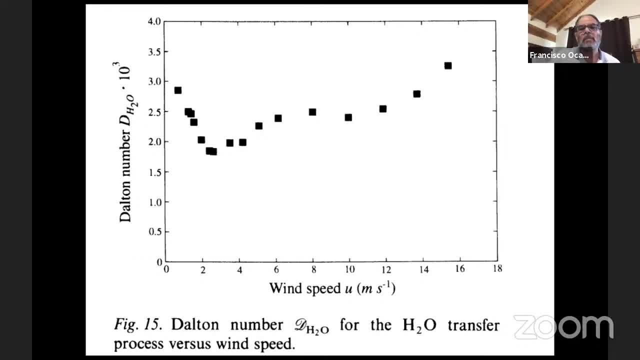 is it a, the, the Patient Magnetic in problem. we're very satisfied with it. the body line, so the model, the, the fins are aligned with each other, but we can see overriding. now we know that co2 is so efficient, we will continue to increase co2 in our produzions基 346 more. continues as we go forward even later over time. whatever we can achieve this, we'll already добute with t св in all our experiments: ion students, but also, but also our products, Emily Flering, ours, because she is the third lead, see, but we have to remember that more than. 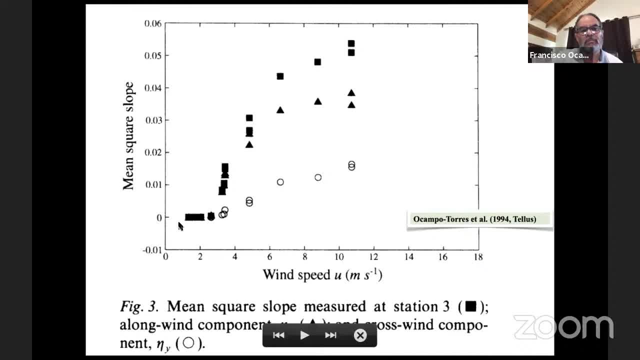 can see in low wind from one meter per second through to three meters per second, apparently, or practically, there were no waves. the mean squares load was practically nil and suddenly increases. when the wind increased up to six or seven meters per second and the increase for further wind speed or higher wind speed is is not as strongly than than for moderate wind speeds. 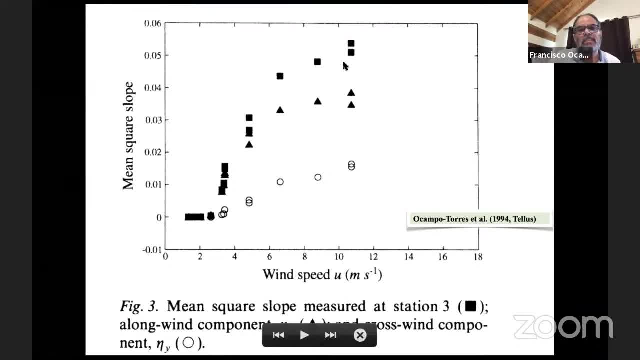 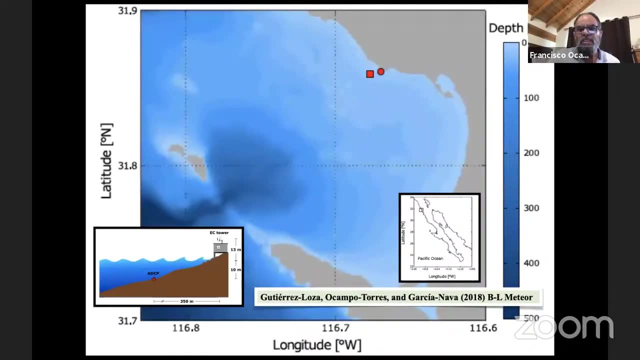 but also is increasing. so what this tells us is that is not only wind speed, but it is important for the exchange coefficient, to determine the exchange coefficient but also the character of the ocean surface waves. with these measurements in the field, in the coastal region in to los santos. 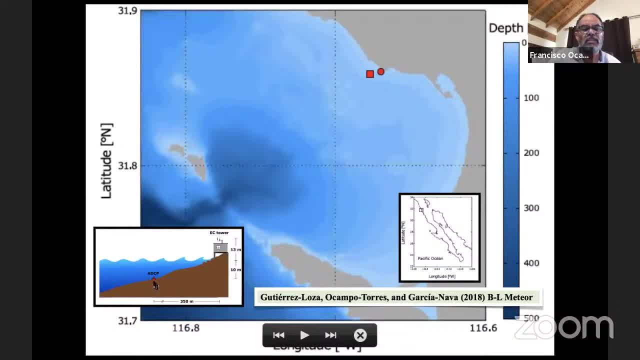 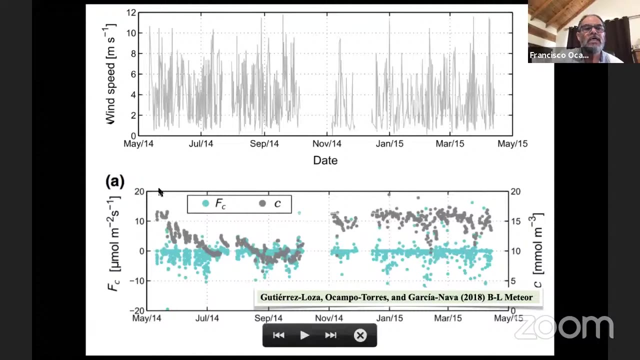 bay, with an adcp to measure the waves, about two or three kilometers from the coast, and we had a ec tower, ediko of eddy, covariance tower, just uh, looking at the ocean like looking at the surf of the of the ocean to estimate the co2 fluxes. so the results are these: uh, the. 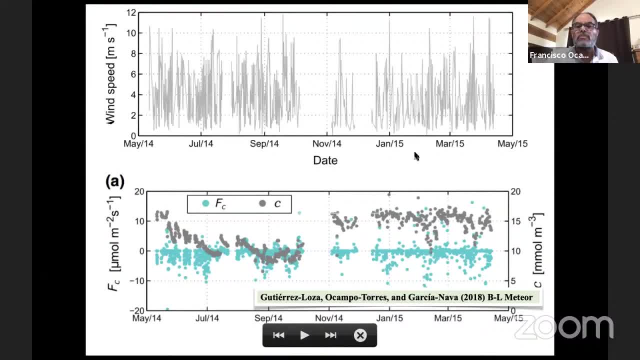 time series of wind speed from may to may 14 to may 15.. sorry, may 2014 to may 2015.. so we managed to estimate the fluxes in a wide variety of conditions of wind speed, from practically zero wind speed to up to 13 or 12 meters per second. 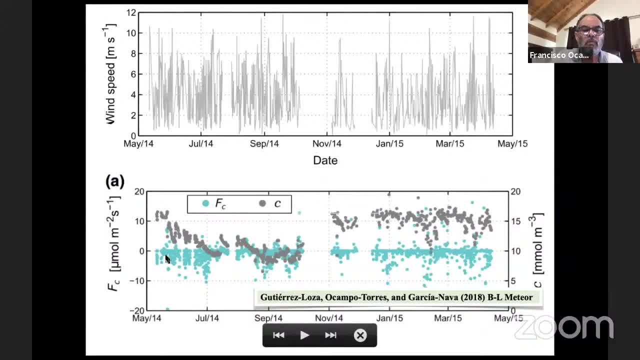 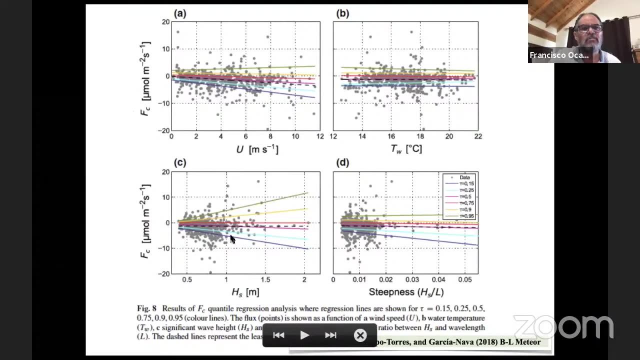 so this is the result for: for fluxes, the, the blue, so the blue or green blue dots, and for c co2 concentration in the air, the gray dots. but it is important here is that we managed to establish a relation between the fluxes as a function of wind speed, water temperature. 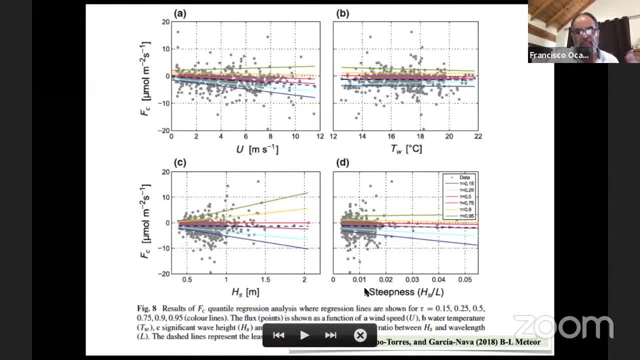 significant wave height and the stiffness of the waves present near shore, and we can. what we we observe essentially is that in not many of the variables there was a correlation between the flux and the variable in considering, except that wind speed, slightly variation and, more importantly, the significant wave height, of course, depending on the quintile quantile regression analysis that we 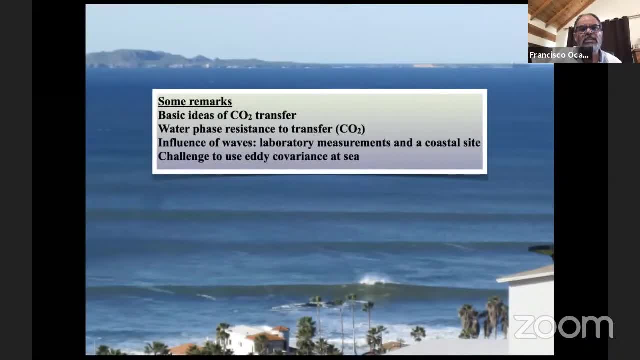 did so with this. uh, we can say that at least we have some basic ideas of the cto co2 transfer between the ocean and the atmosphere. it is already established that the transfer to co2 is weather phase resistance, but we are mostly interested in the influence of waves, so we relied. 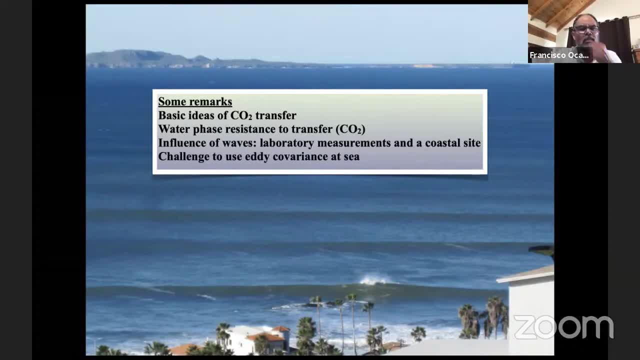 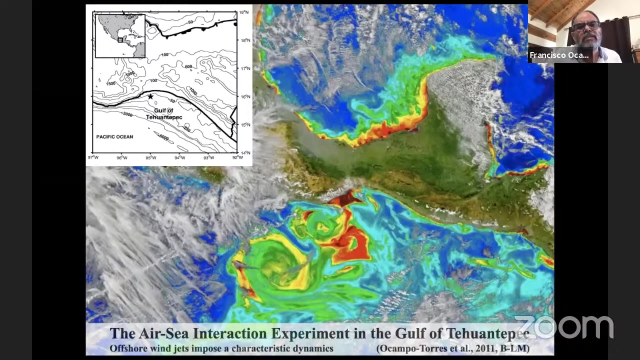 on limits for the. also, but still the challenge is to use the method to the, the valley covariance method, to estimate did in the Gulf of Tehuantepec and in this area there is an offshore wind that imposes a very characteristic dynamic dynamics in the ocean. not only that, we observe eddies around. 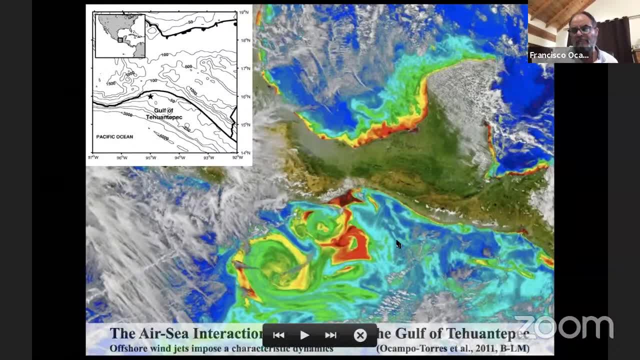 like we can see here by a picture of an idea of the of the productivity that we have in the ocean, but also because the the wind during certain events is very strong, coming from the north, and this wind, which is called tehuano, tehuano event or tehuano wind, generates waves locally. 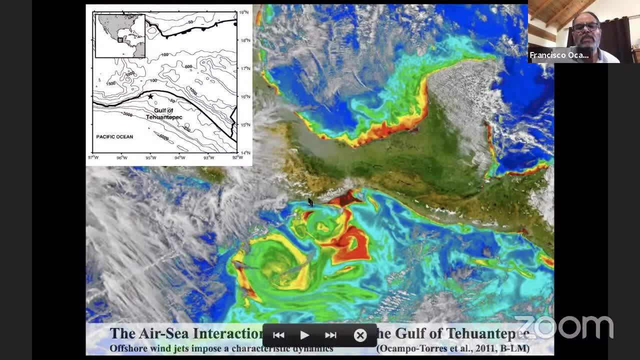 and, as you may know, all the south of Mexico coast receive long waves from the south, from storms in the south pacific or antarctic ocean. so these long waves that coming from the south are directly in opposite direction than the local, than the waves which are locally generated by the tehuano events. so this makes a very particular 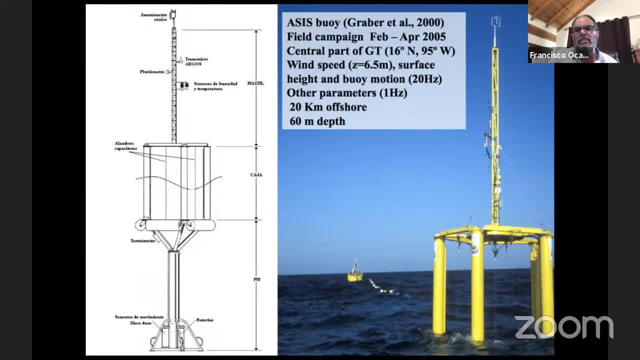 site of experiment for experiment. so we deployed an air c inter and air c interaction spar buoy in 2005 to measure wind speed and surface waves and the buoy motion and other parameters like atmospheric pressure or air and water temperature and so on. with this particular type of buoy it is possible to obtain the through the eddy covariance. 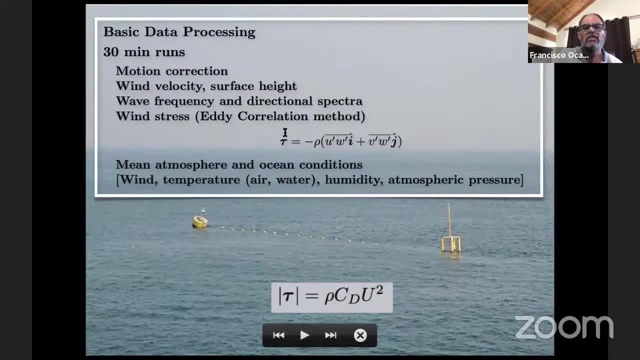 method or eddy correlation method, the surface stress or momentum exchange. so, after the measurements of wind velocity and surface heights were corrected by the motion of the structure, we can estimate the wave frequency and directional spectrum as well as the wind stress, and we can say that the direct way to estimate the the wind stress is this particular 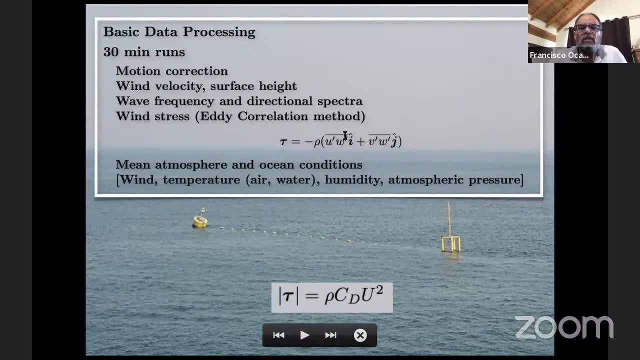 formula which relies on the eddy, the correlation of turbulent components of wind u prime, w prime and v prime and w prime, but as many as i mentioned earlier, the, the surface stress can also be estimated by the bulk formula, just with the mean mean wind speed uh at the square and imposing uh drag. 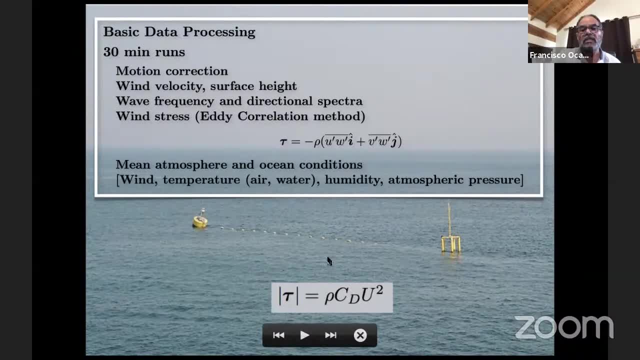 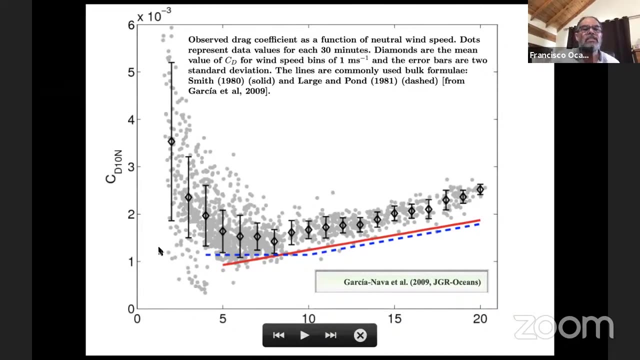 coefficient. so we estimate this directly and calculate this indirectly. we can have a look at this, at the drag coefficient, and try to study the the process. this is one of the main results. we can see that the drag coefficient as a function of wind speed shows also a tendency to decrease with the increase of uh wind speed from one meter per second. 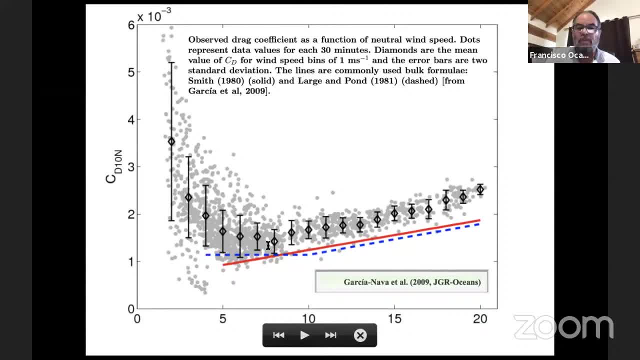 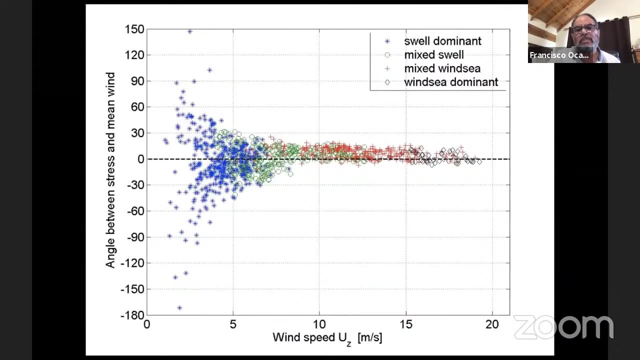 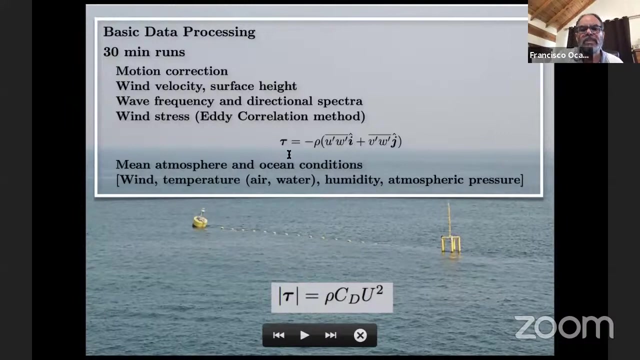 to seven or eight meters per second, and for higher wind speeds the drag coefficient increased almost linearly. so this is more or less a typical character of the exchange coefficient to during low wind conditions. this another another interesting result that we obtain is because we managed to estimate the witnesses wind stress directly. you can see that this is a vector right. 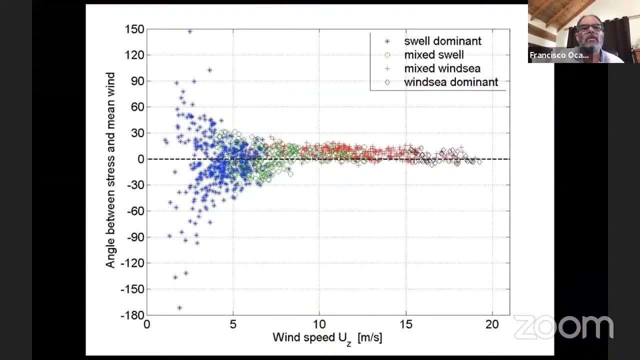 so this vector has a direction and if we compare the direction of that wind stress with the direction of the mean wind, is these results as a function of the wind speed? but we can say here is that during low to moderate wind conditions the direction of the wind stress is not aligned with. 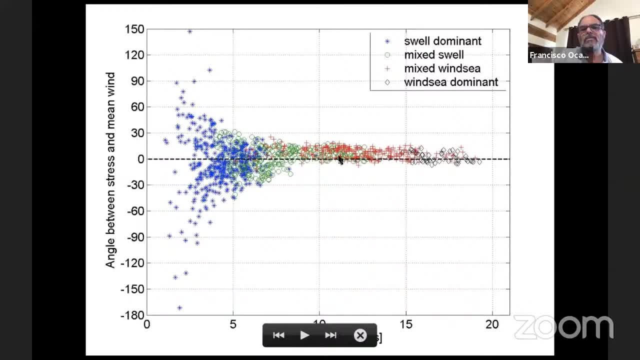 the mean wind. it is aligned only for moderate to high wind conditions. this is really important because if we use the bulk formula in a numerical model, we always assume that the wind stress and the mean wind are aligned, because it is only considered the intensity or magnitude of the wind. 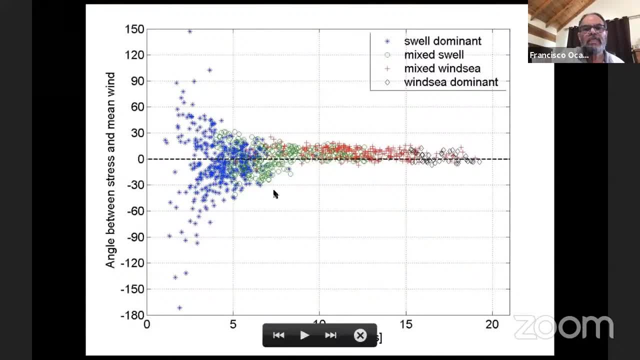 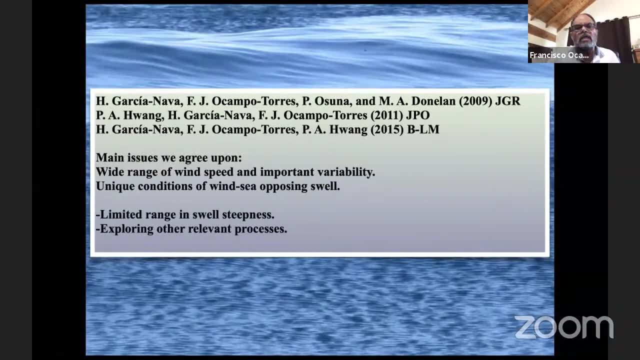 stress, but measurements now reveal that this is not the case in many, in many occasions. so several research documents were obtained from that experiment and there are some main issues that we agree upon: that we obtain a wide, wide range of wind speed and we also observe a very 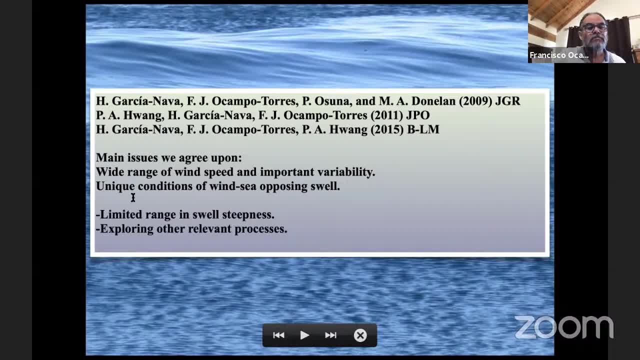 important variability in our results. so we can see that the wind speed is very unique with conditions of wind sea opposing swell, which is the long waves coming from distant storms. but the important point here is that the swell stiffness in the experiments was in a very limited range, so we need to explore also other relevant 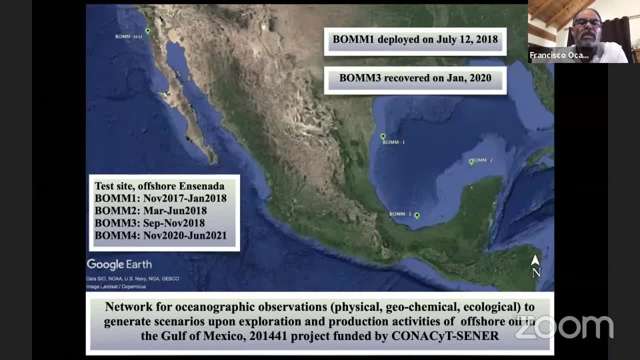 processes in the exchange. so we have the opportunity with a project by conacyt center, the big experiment sigon, to develop and build boyas meteorological and oceanographic spar buoys. we have some tests in the santos bay and we deployed three of them in the gulf of mexico. 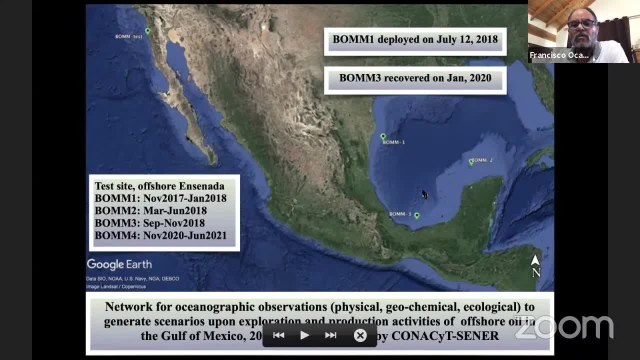 unfortunately not. the three of them were working or functioning simultaneously. we deployed the first one in july in 2018 and later on the the other two, and at the end we recovered the last one in january 2020. but at least we have some. 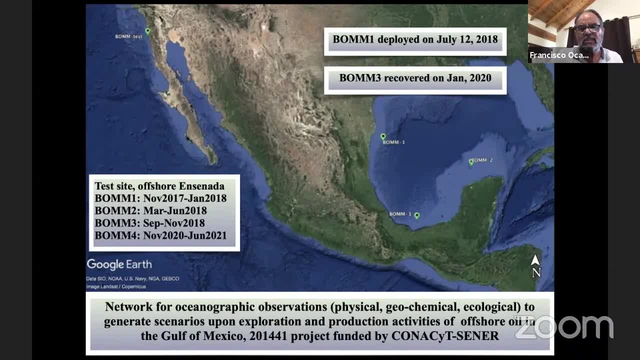 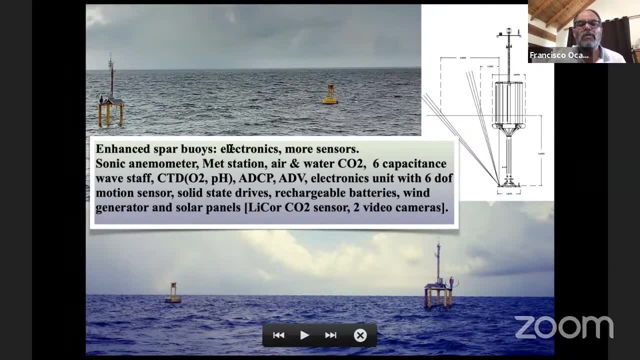 results of two of the buoys simultaneously. these buoys are enhanced spar buoys dealing with more electronics and more sensors than before, and one important thing is that the electronics and the connections of the buoys were developed in our laboratory. the buoys had a sonic anemometer, a metastation. 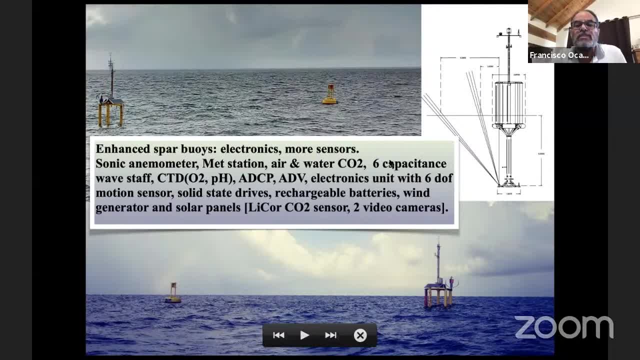 and we measure co2 in air and water. and also they have six capacitance wave staff. besides ctd for with oxygen and phd sensors, an acoustic doppler current meter and adb and within the base of the structure, within the electronics, there was also a very fine 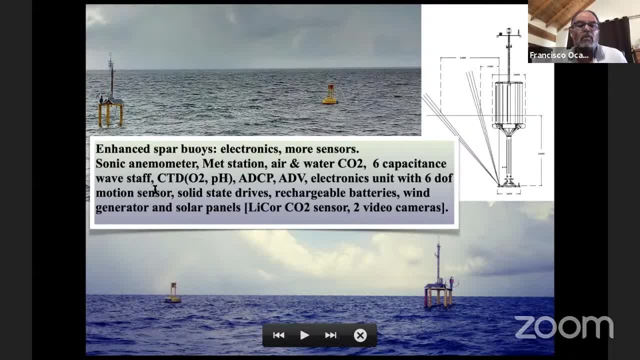 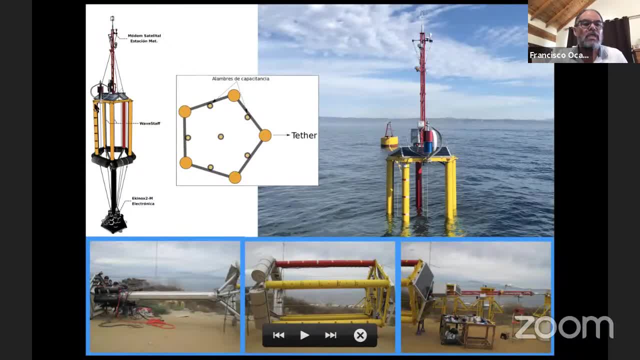 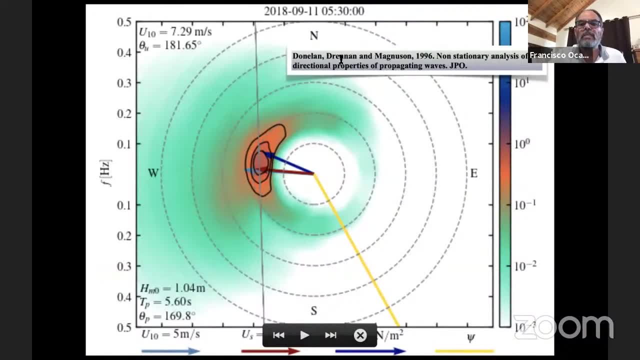 sides of this pentagon, which is the pentagon, essentially, is given by a south and west. so this plot, this particular plot, which is the results from a half an hour data center, or starting in 5, 30 of 11, no, yes, 11 of 11 of september in in 2018, 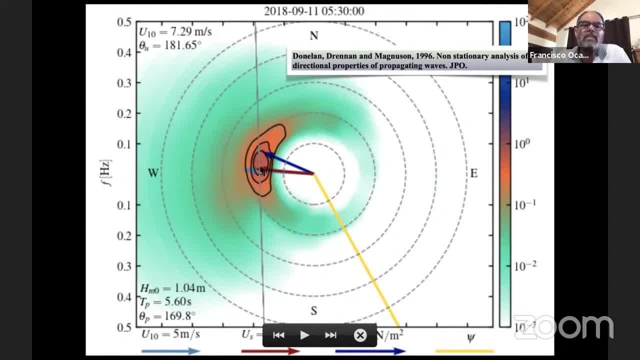 indicates that the main wave energy where was traveling to the west and the waves spectral peak was about 0.2 hertz in frequency. the result from this analysis can also provide us with the wind speed, which is the the blue arrow, the stocks drift, which is the red, and the stress, which is the blue, dark blue arrow. 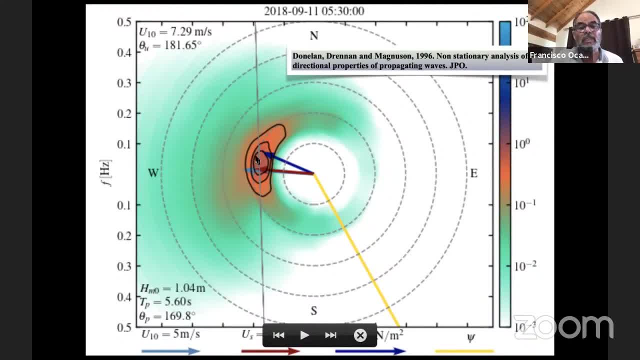 so in this case, the waves were traveling towards the west and the wind and the stress appeared from a very vertical próxima mode and the wind came in through a thickassemble and the stocks drift was also directed to the to the west, but this is not always the case. 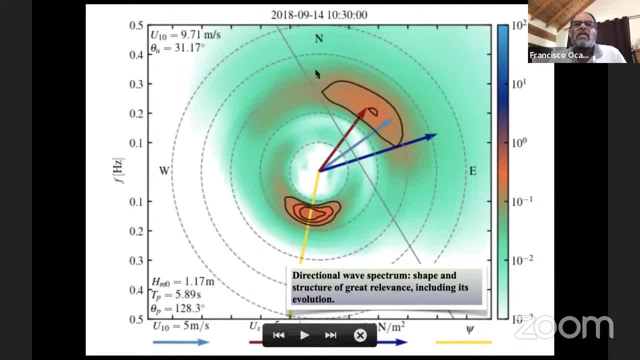 we obtain results from this one- uh, the 14th of september at 10: 30, where we have two systems, two wave systems and, of course, the. the results of wind speed and stocks, drift and stress are with very different direction. so this is very interesting results and we need to. 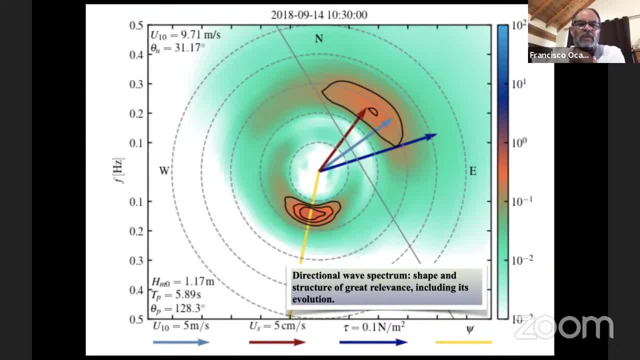 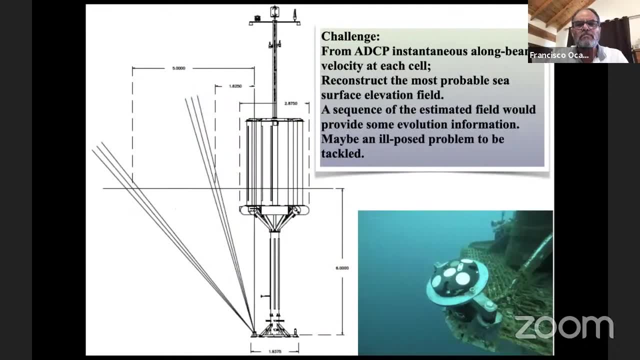 to further analysis, analyze them in order to establish a better relation between the ocean surface waves and the wind stress. besides, as i mentioned, we have an adcp at the, at the base of the structure. looking upwards like, these lines are sketchy and this is a picture of the adcp. 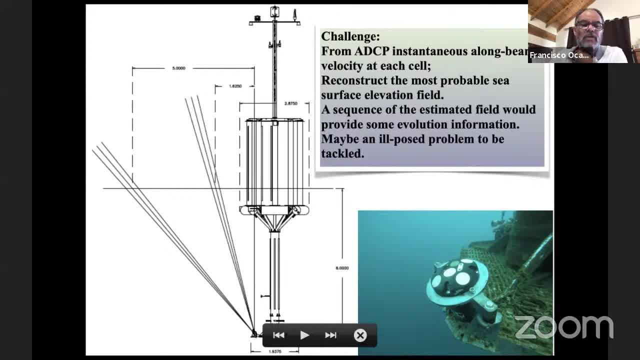 and this is a picture of the adcp, and this is a picture of the adcp and this is a picture of. the idea is that the this sensor has five acoustic beams and in each acoustic beam we can estimate the along beam velocity of the fluid particles in every cell, from the bottomless. 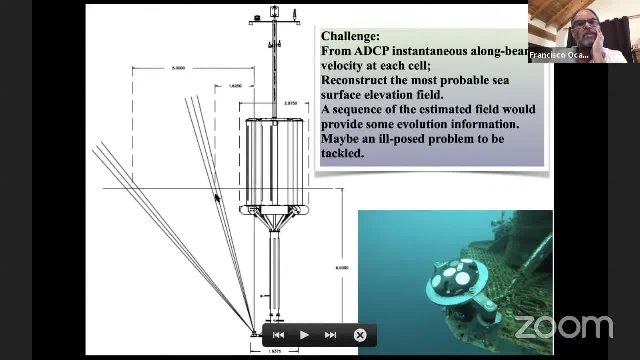 structure right to the, to the surface, the. the sensor was sampling at 16 hertz so we have, at 1, 16th of a second, a snapshot of a long beam velocities. so we we need to reconstruct the most probably surface elevation field from those from that signal and from a sequence of the estimated field: surface field. 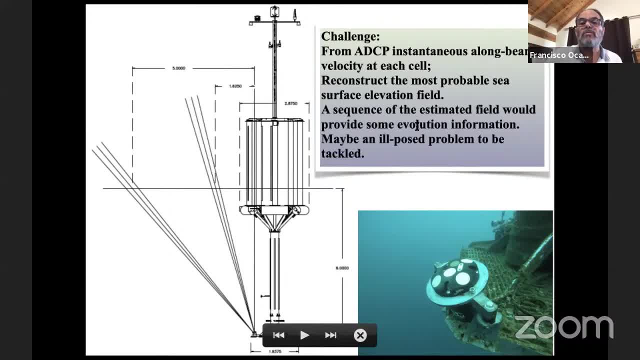 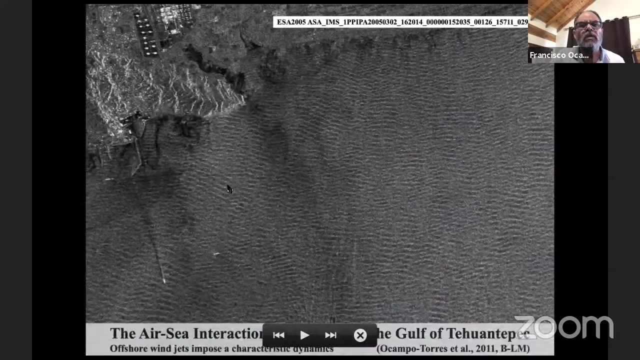 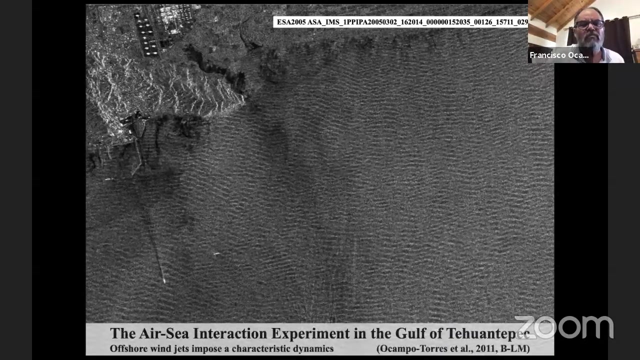 we. this will provide some evolution information. this is a very interesting problem. maybe it's an ill-posed problem to be tackled in order to use the amount of information that we have to obtain from the adcp and trying to reconstruct the sea surface evolution. so another topic of interest and looking at the ocean surface waves now from very far above. 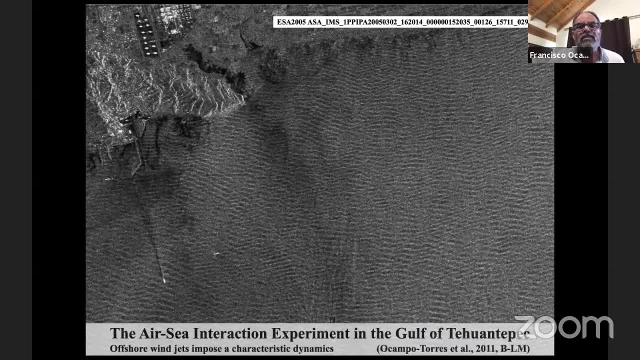 is using a synthetic aperture radar. this is an example of an image obtained also during the experiment as well, in the hoof of taiwan, tepec, and here we can detect the coastline, and this is the port of salina cruz and the port of pemex right there. 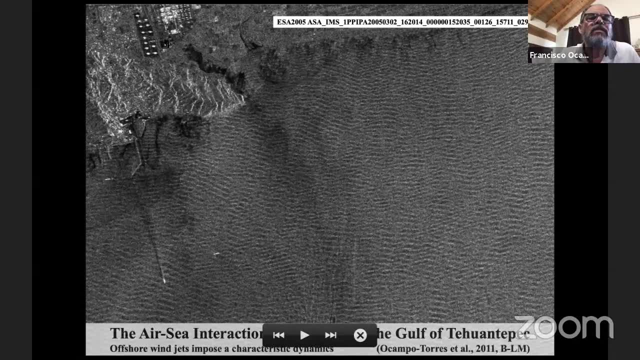 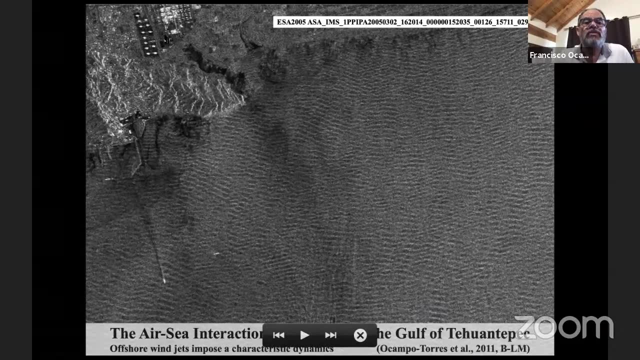 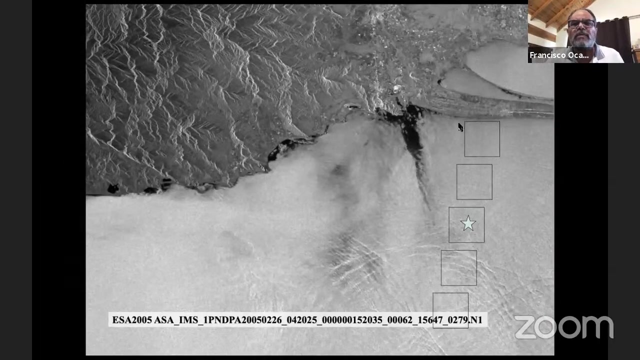 and also very distinct. we can detect the oil refinery and storage of pemex in that region. what is important here is that we can clearly detect some uh features that tells us that there are waves present. right, i hope you can see. they see them. and we did analysis of sub images in a similar image from synthetic up the radar extract. 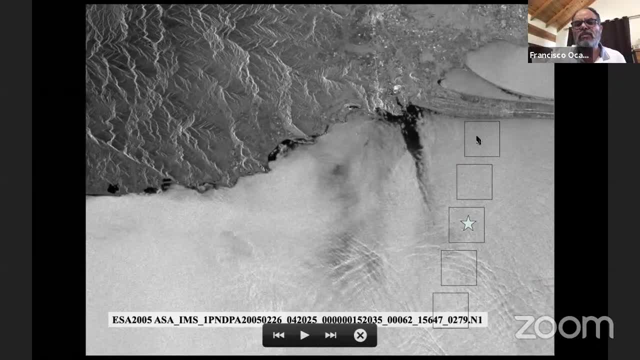 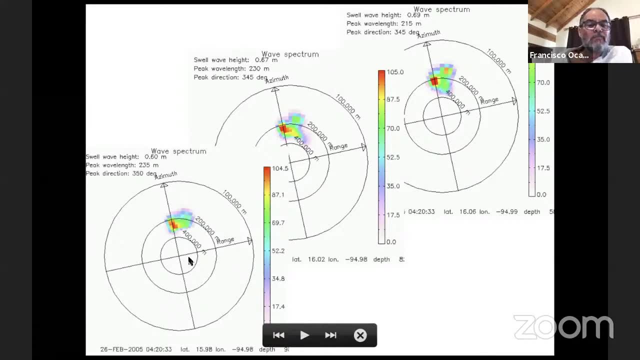 information from these five squares to estimate the directional wave spectrum and we plot them again from similar to the directional wave spectrum that we showed before. in this case we have a wavelength 400, 200 and 100 meters and the colors are also energy or the energy density for from the spectrum. so in this case we can detect the evolution of the waves. 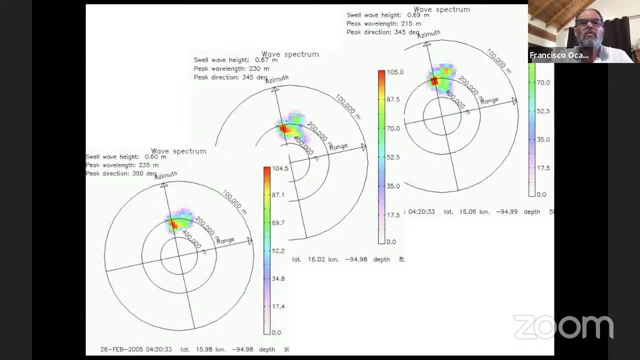 in terms of the directional wave spectrum when they travel towards the coast. so we can see here that in the far away square or sub image, the waves can be detected only like traveling to the azimuth direction, which is practically 10 degrees off north. but in the when when the waves are getting closer to the 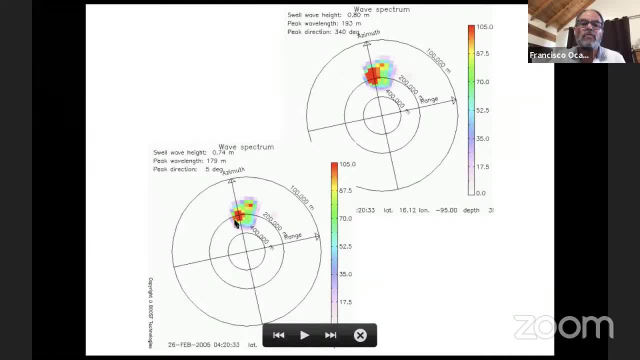 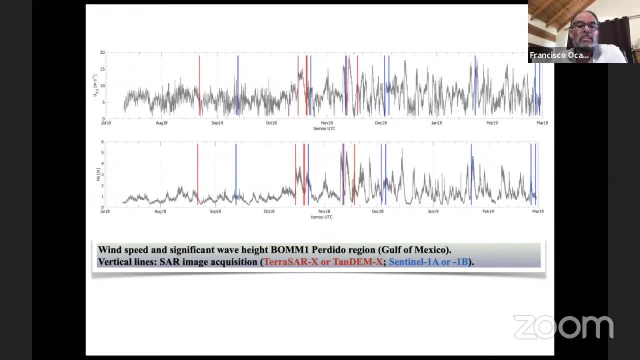 coastline, the variability increases and we even obtain or detect two wave systems. so this is also a challenge in well. before commenting about the challenge, let me show you some other results in the group for mexico for newer satellites, for newer synthetic activity radars from satellites from the german laboratory and from the. 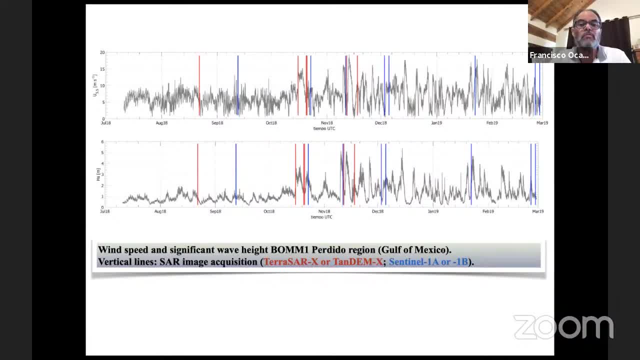 european space agency, and this is because we have at the same time measurements from bomb one at the perdido region in the gulf of mexico. so the time series that we are showing here is the wind speed in the top and significant wave height as obtained from the buoy, and the lines are when we obtain. 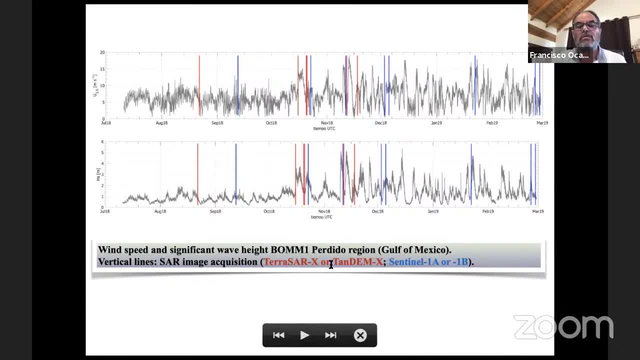 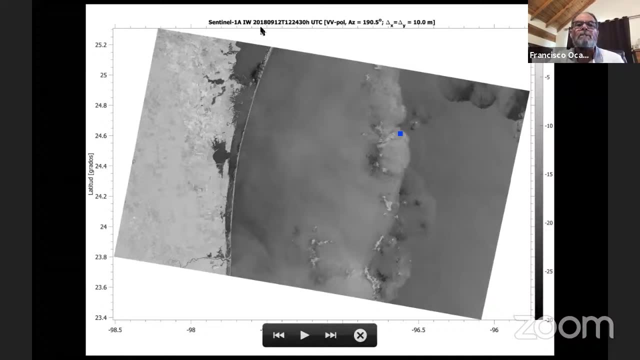 images either from teras rx or tandem x or the european space agency satellites sentinel 1a or 1b. just as an example, i'll show you a an image from 2005 that comes from central europe for us, so that was in september 2018 and the buriti. 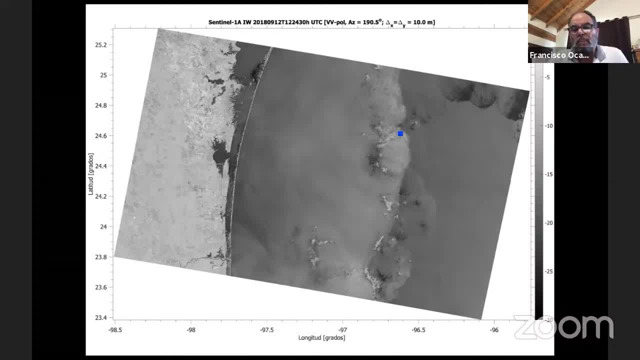 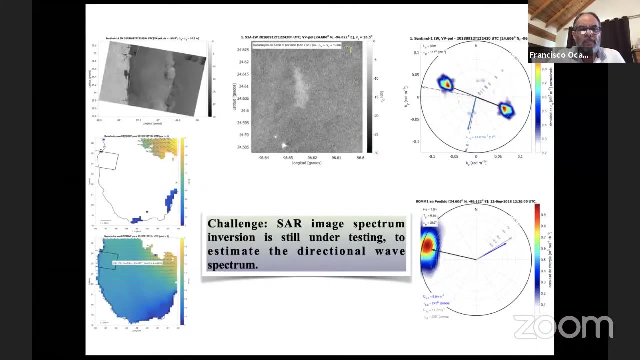 from central europe folder first changed to theaign the blue square, so the blue financing usingnentome was used, the gray circle to be represented as the large vertical projection with the blue square from the cosmonaut. but this is only the same action images in that particular region and we estimate the image spectrum from. 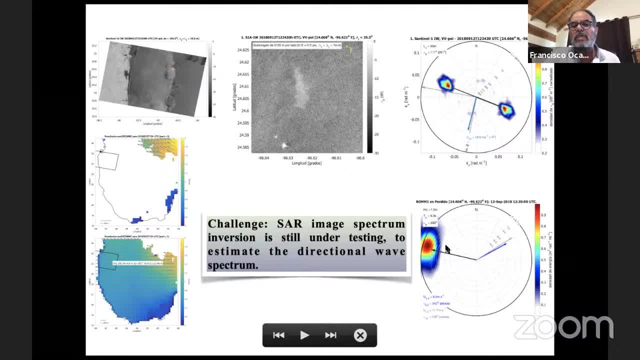 directly the sub image, but we can also estimate the directional wave spectrum from the buoy. and this is the challenge because we are- we are still under testing and building the code, building the model to retrieve the information from wave spectrum, from the direct information of image spectrum obtained. 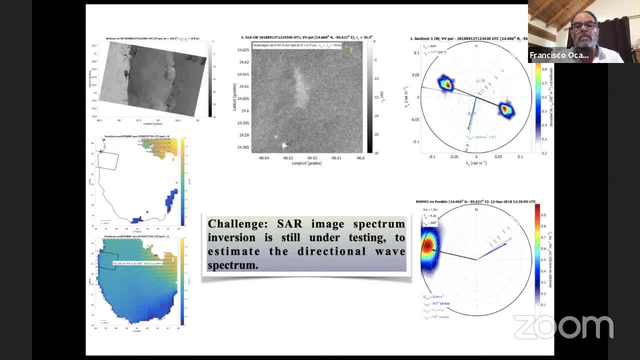 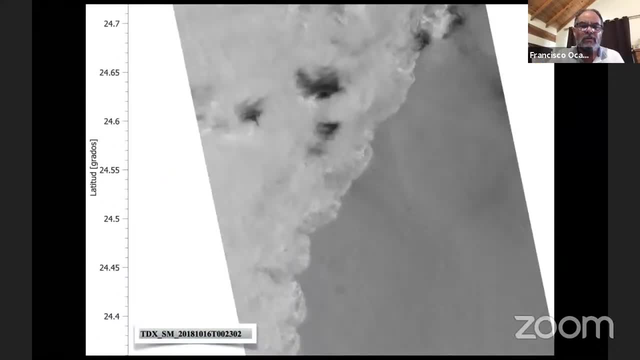 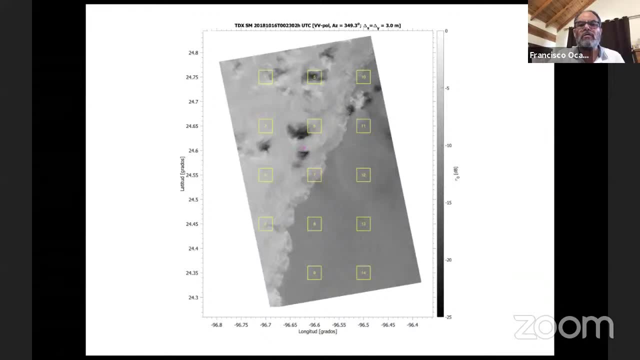 by a synthetic aperture radar. so this is one, one problem that we still- we are still working on it, and another. another example is the 16th of October 2018, when there was also another cold front. in this case, at the time of the SAR image acquisition, the buoy was in this magenta cross. 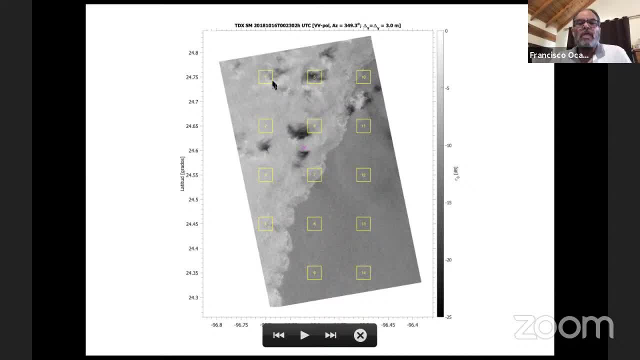 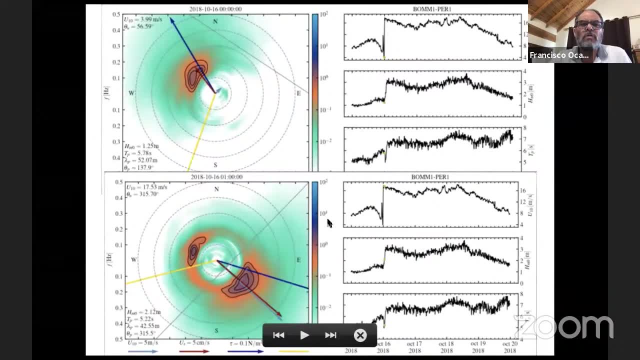 but we managed to estimate wave information in all these sub images and we can just show you the results of the directional wave spectrum from the Buoy just before the front gets Eneridences over the actual buoy. so the wind speed at this particular region is at this particular time. 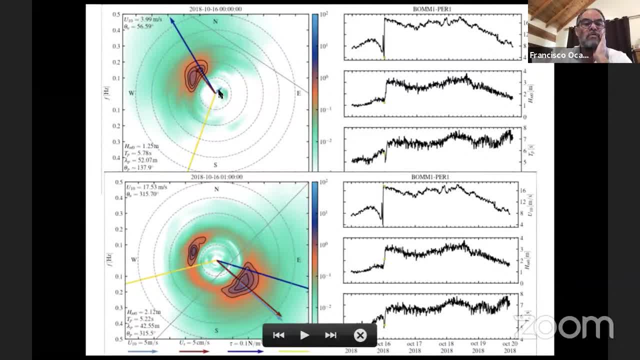 is very low, almost four meters per second. so the the light blue is the wind speed and the stress and the stock drift are these arrows. and just when the actual front passes by the buoy, the wave conditions changes dramatically. and it is, and there is only a few hours or one hour difference between this signal to this. 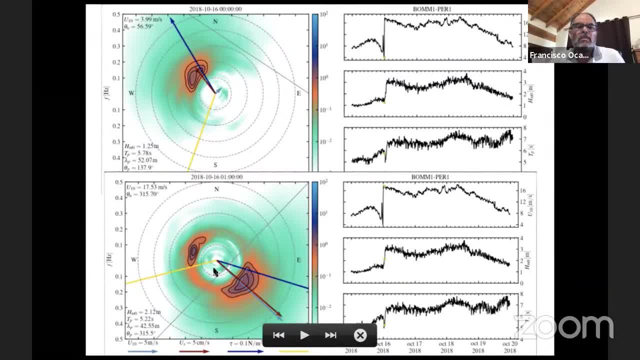 signal and the results. and the wind speed is now very intense- 17 and a half meters per second- and of course, the wind conditions are very different. so the wind speed is very high and the stress and the wind speed are very different. and what is more important is the 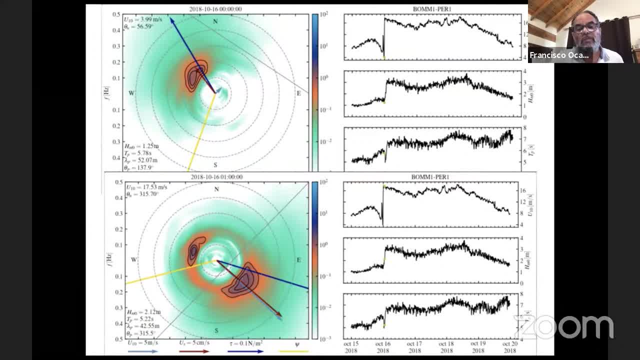 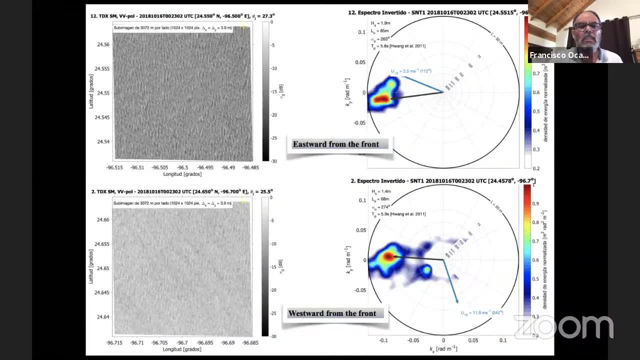 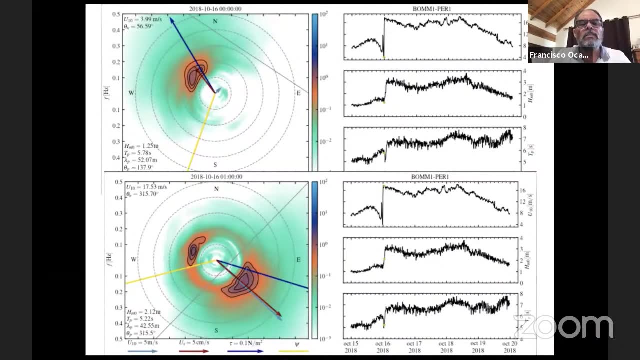 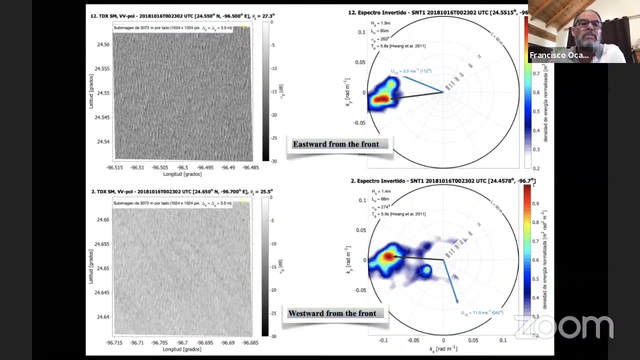 exchange coefficient, the momentum transfer and even the stocks drift are rather complex and difficult to to estimate. and from the image. so this is, as a function of time, description of what happens, uh, right in the station where the buoy was, but for that particular instant, when the when the image was acquired, eastward from the front, we estimate this wave spectrum from the. 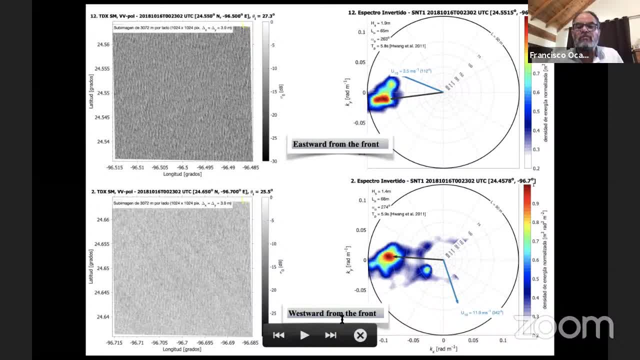 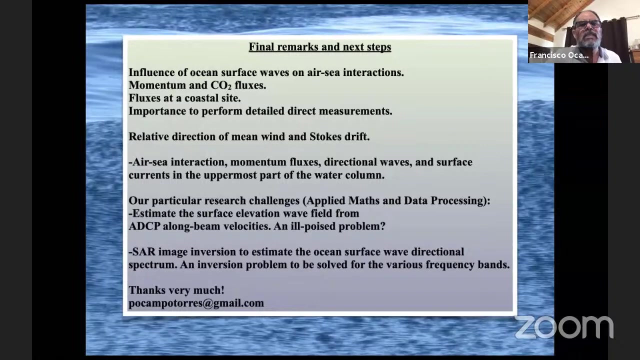 sar image and westward from the, from the front, we estimate this one. so this, this is uh work under programs we need to to to work on details of the retrieval of the directional wave spectrum from the image spectrum and look at the. so that's final remarks and next step. so we just showed that there is important. 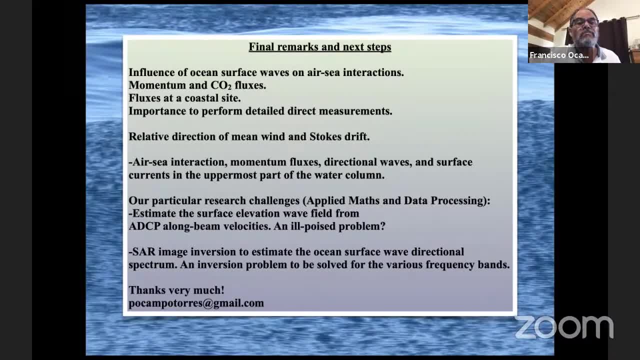 great importance of the influence of the ocean surface waves on the sea interaction. These ocean surface waves influence momentum and CO2 fluxes. for instance, We did some measurements and show results from fluxes at a coastal site and we are facing and we are dealing with the 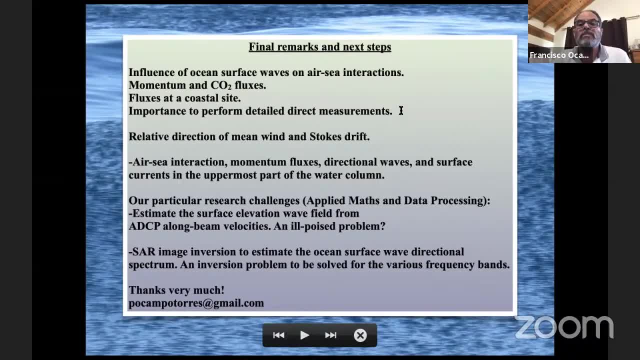 detailed direct measurements with sensor in the coast, but we would like to deploy these type of sensors in the buoy. We still don't have the CO2 turbulent fluctuation measurements in our world buoy but we are working on that. With this type of result we can estimate very neatly the relative direction between. 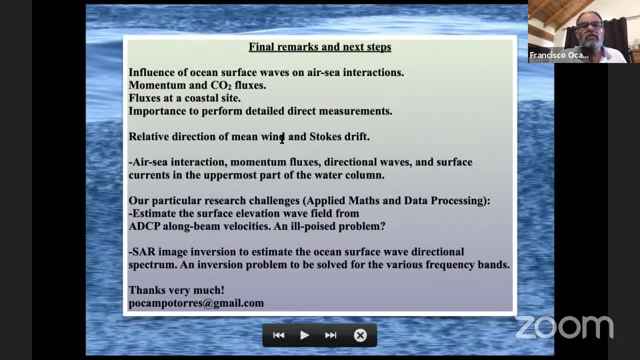 mean and clear waves, wind and stop drift, which here, which is rather important for um oil oil transport or sargasso transport or any particles on the surface. motion there's interaction, momentum fluxes, directional waves and surface currents in the uppermost part of the water column is one of the main interest. 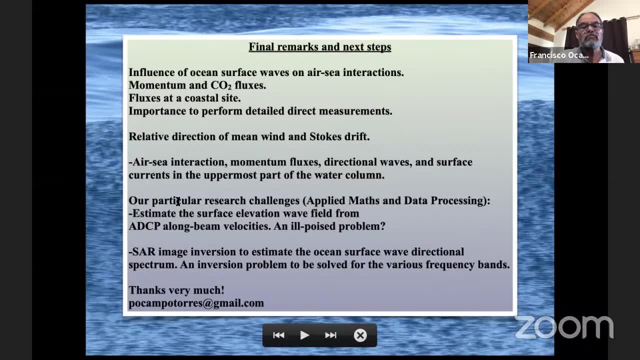 in our research and our particular research challenges, mainly associated with applied mass or data processing, is to estimate the surface elevation wave field from the adcp data, essentially along beam velocities. you know, you know cells, uh, as a function of the of the depth, and we anticipate that this is an ill-poised problem. another particular chart challenge is 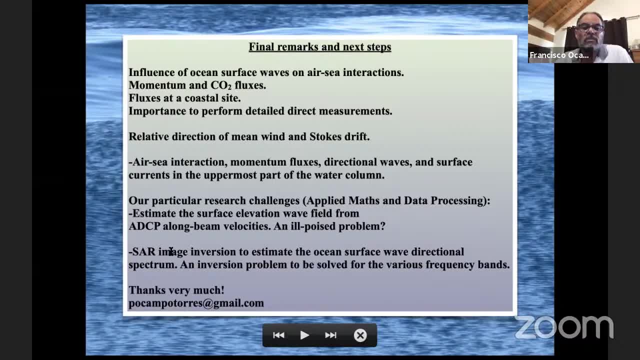 the sar image inversion. in other words, strictly speaking, these are image spectrum inversion to estimate the ocean surface wave directional spectrum. we would like to reach an inversion scheme and the problem has to be solved for the various frequency bands that we are using, essentially x-band from the german satellites and c-band from the european. 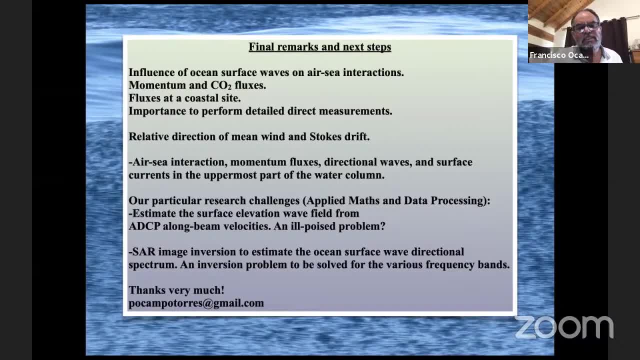 space agency satellites. and with this i finish. thanks very much for your attention and welcome welcome any comment or questions. uh, thank you very much uh for this interesting talk. uh, dear audience, as you see, at the bottom of your screen there is a chat where you can write your question, or you can raise your hand, that yellow hand, and your microphone. 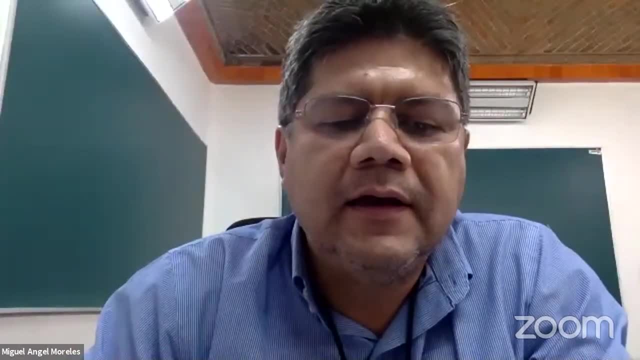 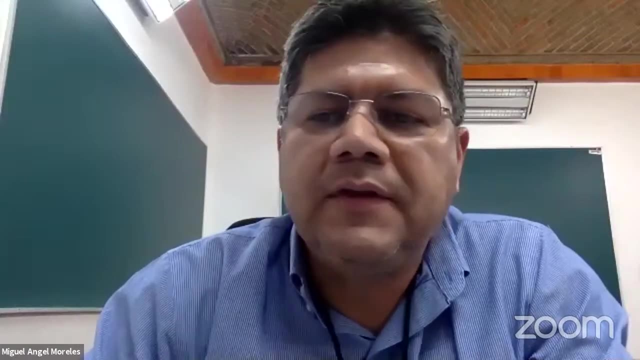 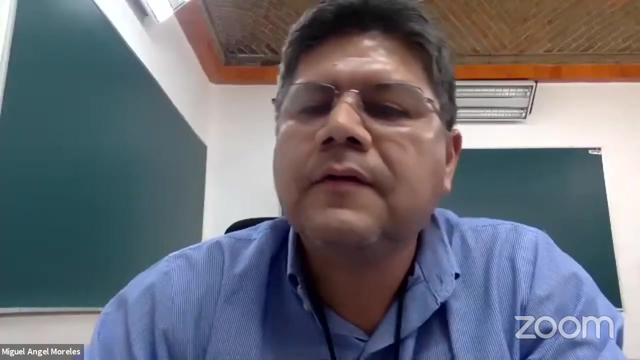 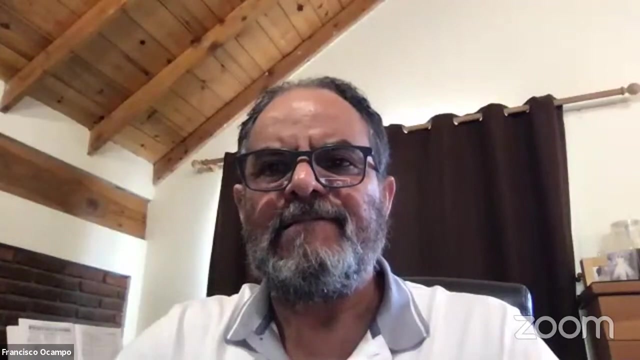 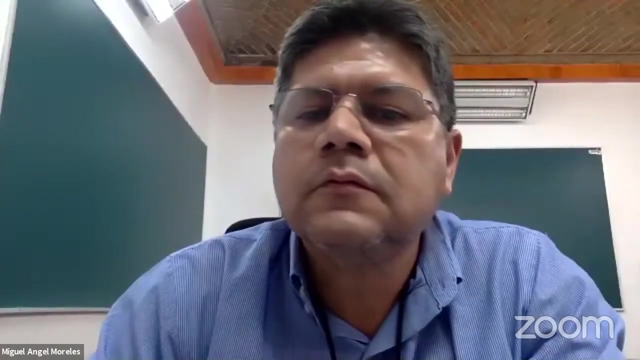 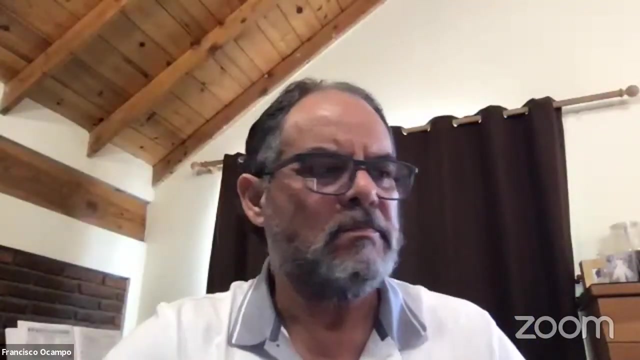 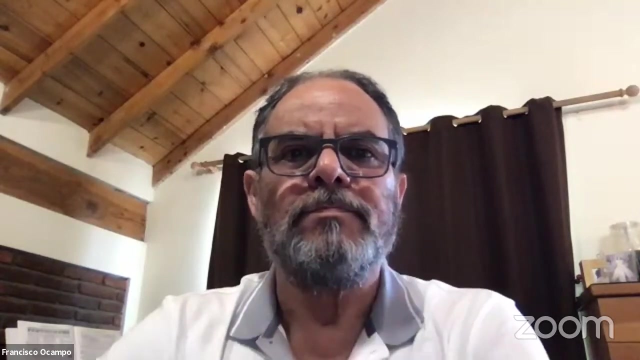 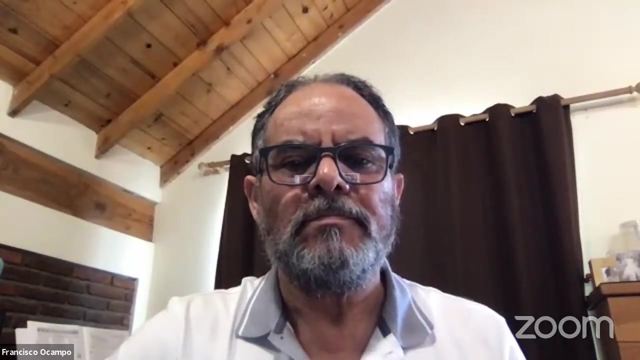 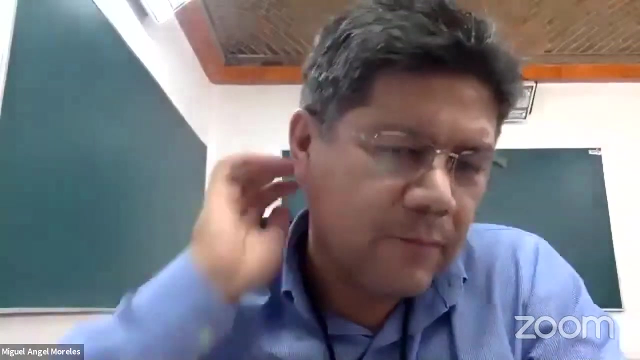 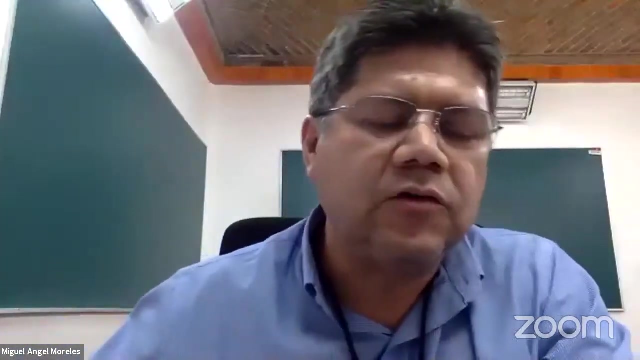 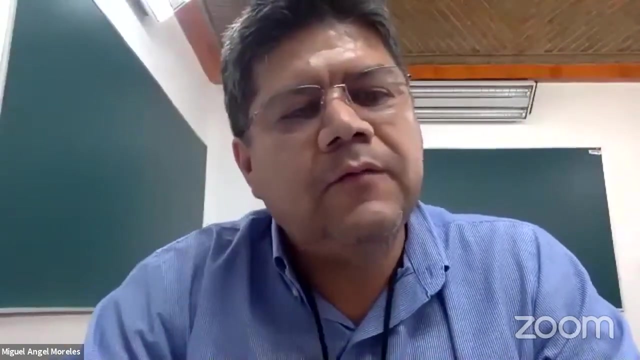 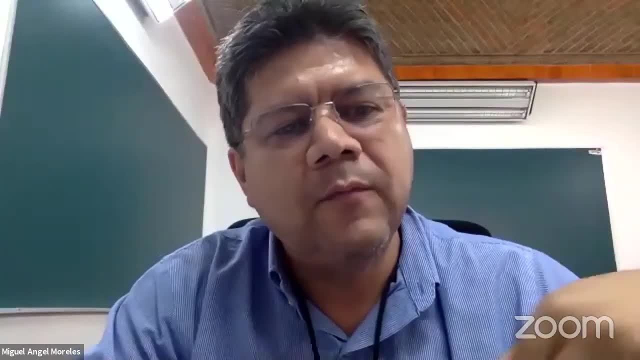 an auxiliary behavior and if in the first figure it was, it was clear at the it wasn't. the grass was the curve was decreasing, reached a minimum and then was increasing. but in the situation the graph was was decreasing, reached a minimum and then was increasing. but in the situation 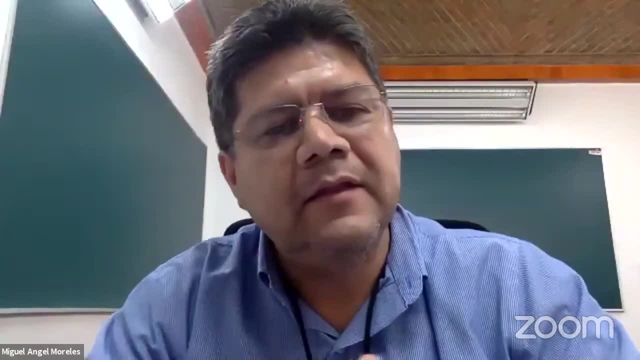 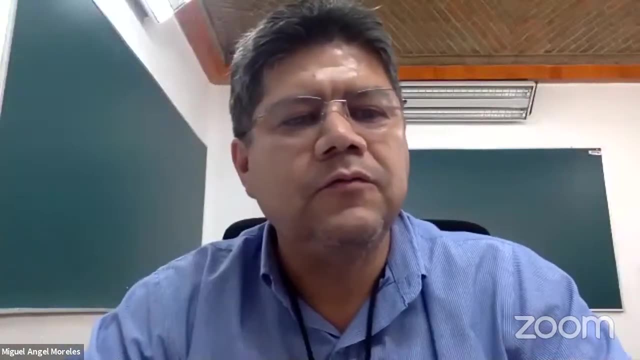 but in the second figure you have at the beginning the same behavior, but then there was a kind of oscillatory behavior. Is there a physical reason for that that you could comment? Yes, I'll show the picture again. Yes, 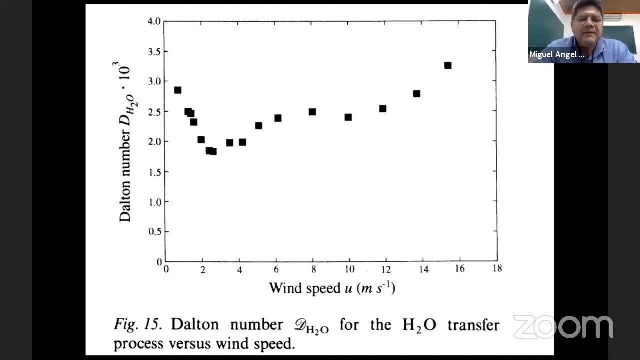 So this is for CO2?? Yes, and then in the second one there is this kind of oscillatory behavior that looks quite interesting. Yeah, yeah, It is quite important, because we noticed that this increase is suddenly for higher winds than three meters per second right. 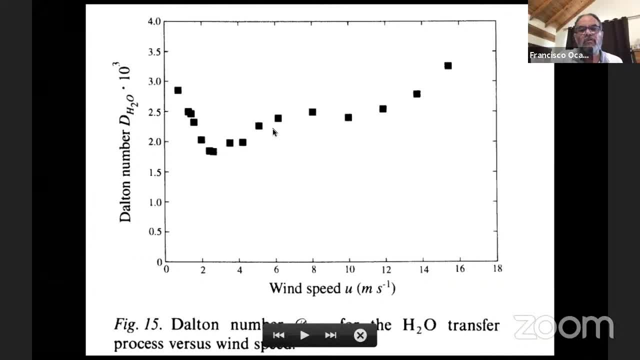 But then in the wave tank, with three, four, five or six meters per seconds, the waves start to break right, And then for six in wind speed, conditions between six and 12, there was apparently- I mean avoiding this- dot. 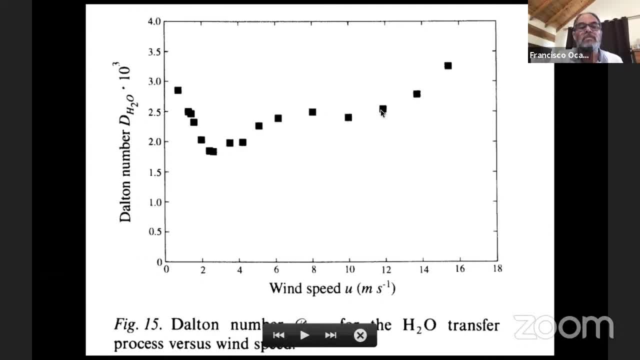 you could see that it is a rather constant Dalton-Nagy Number for winds between six and 12 meters per second. okay, And this is due to the wave breaking that this wind imposes, And for even higher wind conditions, the wave, of course, break mainly. 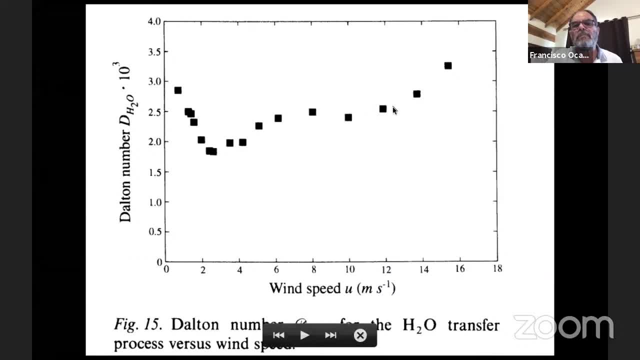 well, the waves are increasing and mainly breaking, or you could say there is micro weight, micro breaking under these conditions. But for higher winds there is a strong breaking And essentially the waves break very intensively in the end of the tank where there was a kind of beach. 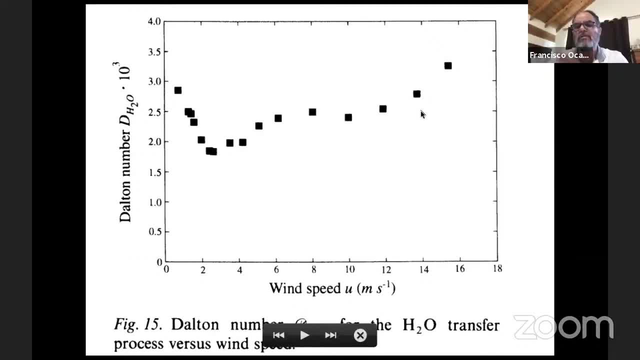 So, yeah, there is a physical reason. no, There is microwave breaking all over. these conditions of wind speed And strong breaking increases suddenly the Dalton number or exchange coefficient for evaporation. Yeah, We thank you. Is there any comment or question? 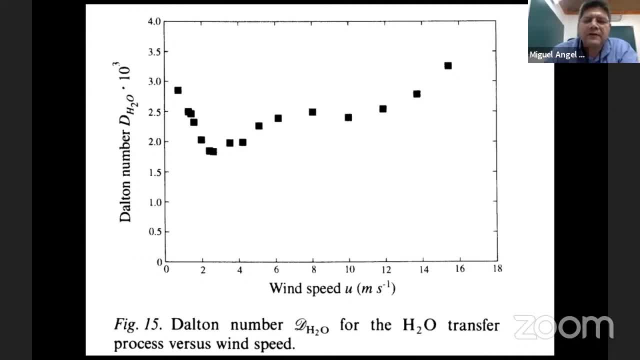 Well, I have many, but let me just ask another one. Okay, There is a lot of data generated in these studies. Is there anybody interested? Is that data available? Yes, definitely, We welcome any collaboration So we can easily can provide with you with the data. 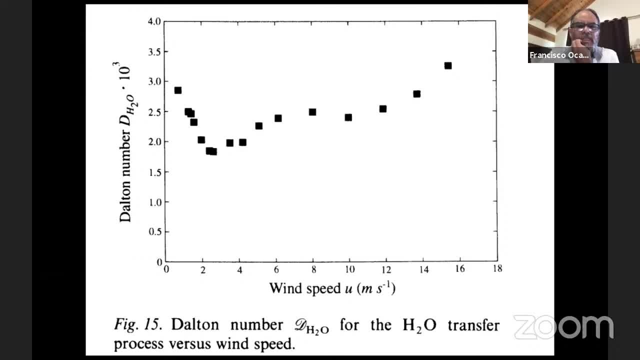 And, if needed, we can collaborate and do some things in our group and some other things by any other possible collaborator. Yeah, We are open to collaboration and definitely share. We can share the data, Thank you, There is Fabricio with a question. 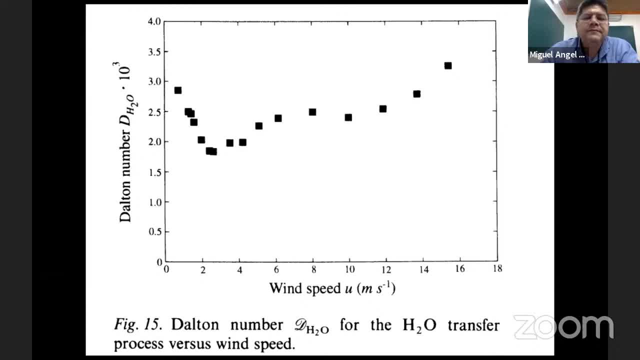 Please open his microphone. Hello, Good morning, Fabricio. Cheers, Good morning, Cheers, Good morning. I have a question. We know that from centuries the humankind has been modeled ocean wave spectra From the point of view of a physical oceanographer. 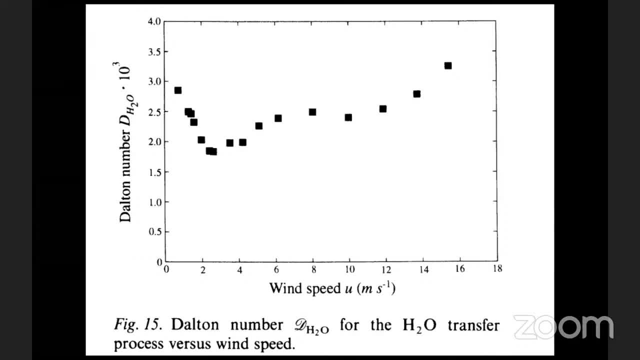 what do you think is the state of the art of this modeling about ocean wave spectrum? Well, if we consider modeling the ocean surface wave spectrum, there are two things right. One is to have a specific model spectrum, like Pearson-Moskowitz, like John Swap and so on. 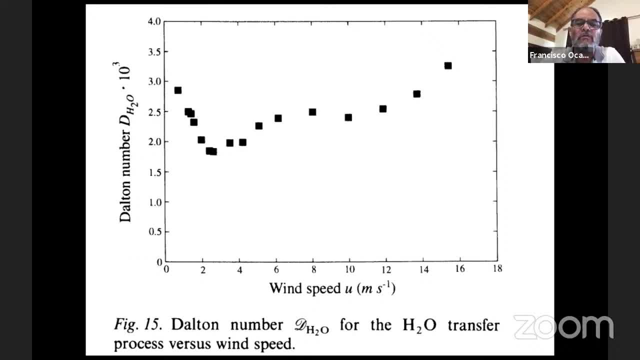 But, on the other hand, it is the subject of numerical uh model to predict the ocean surface waves or the ocean surface wave spectrum. right, Okay, So what is your question regarding the typical model spectrum, like John Swap or? 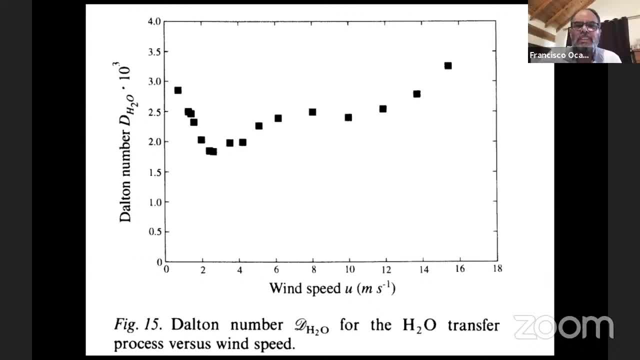 My question is more about the data- Yes, data, Because I know there are many models, like you have said before, but more on numerical, Uh, numerical modeling, for example, because you showed us many um, spectra, um that comes from data. 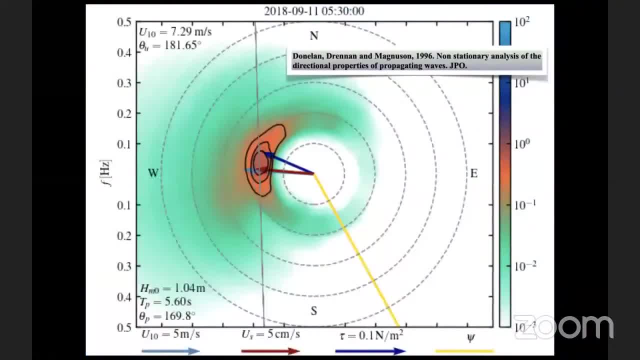 So I would like to know more about this modeling and the state of the art about this. Okay, The spectrum that I'm showing now is directly from the data that we obtained from BOM-1, the buoy in the Gulf of Mexico And uh. 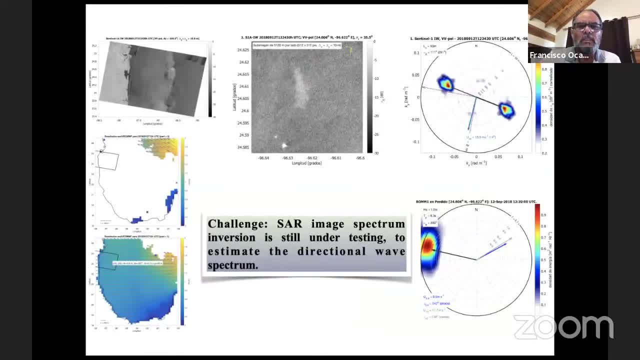 Okay, Mm-hmm. So the more modeling you make with numerical data, then you can find a kind of universal spectrum. Am I right? No, no, no, no. Ah okay, Universal spectrum is useful, but it's only very idealistic. 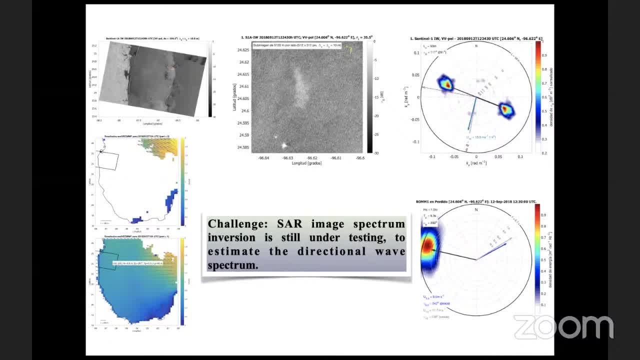 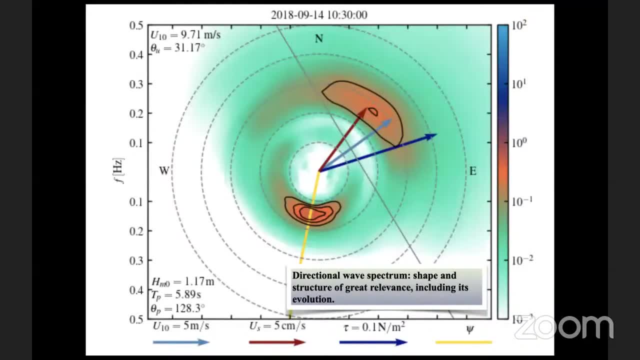 Ah, okay, That's why I'm very interested in showing you direct results from measurements like the one we see here, right? Yes, Because at one time we have this kind of a spectrum and suddenly we changed everything. So instead of one wave system, 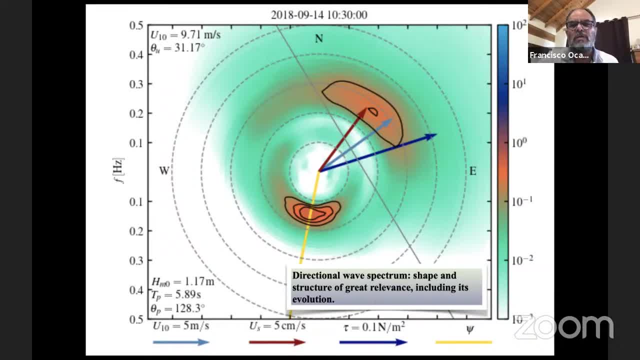 now we have Okay, And all conditions are rather different, you see, So it is not Unpredictable, not possible to have a universal wave spectrum. Ah, okay, okay, in this region We can show it clearly here, right? 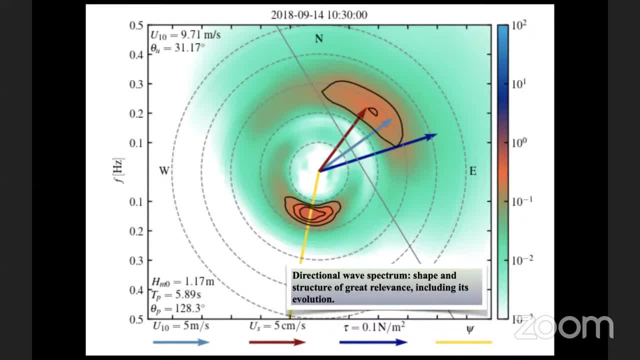 Okay, So there is a lot of work to do with data in order to find a specific spectrum just for a certain region in the ocean, Mm-hmm. Okay, So thank you very much. Thank you. There is a question by Joaquin Delgado. 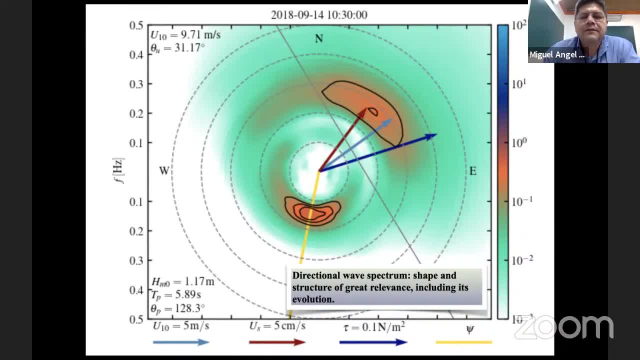 Please open his microphone. Okay, Thank you. Very nice talk. Thank you, Francisco. I just want to know if there are some kind of rough models, not with such detail, but just to have a global view of the interaction of the ocean and the air. 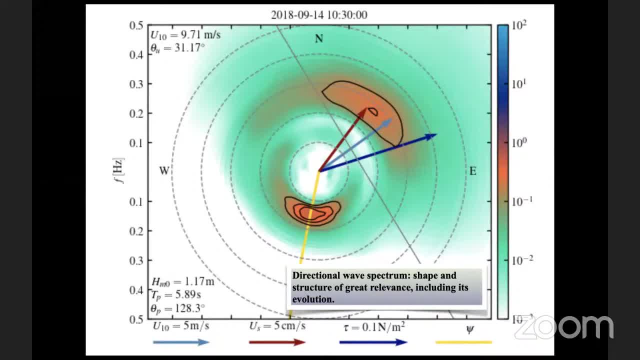 And I'm thinking about, like Raleigh-Bennard, model convections, of course, with the appropriate modifications. Can you give a basic reference on that? I'm afraid not. I know that there are models and, as you said, 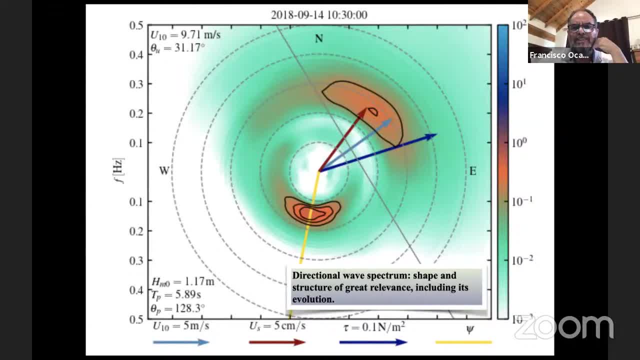 are focused most on the global scale And what we want to stress with this type of work and this talk is that, behind or before those global models, we better understand more detail of air-sea interaction processes, because it is within the, we could say. 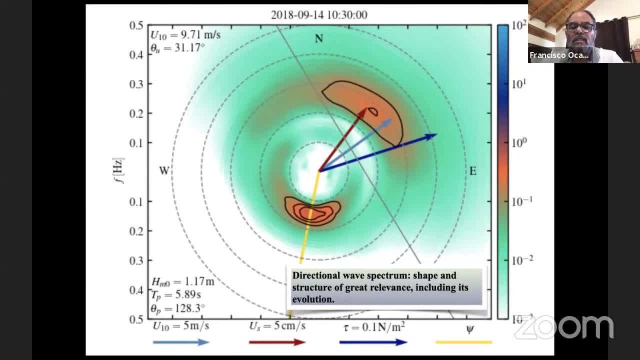 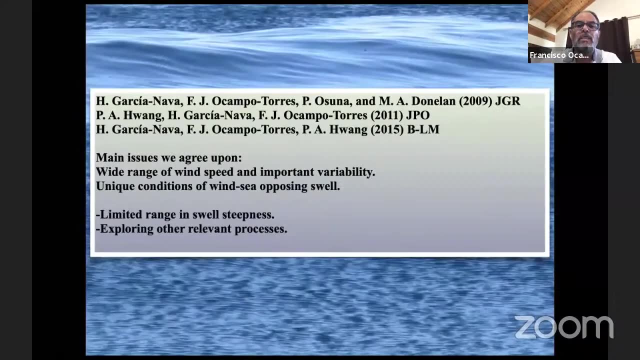 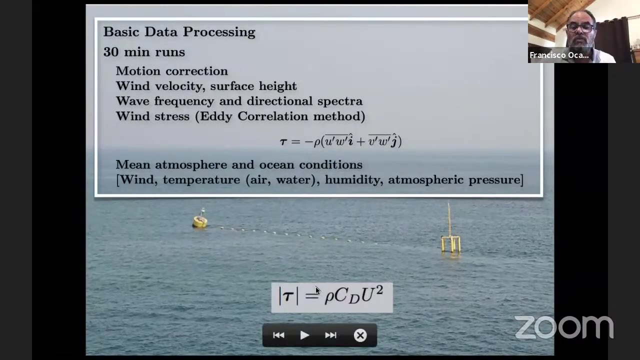 micro scale, that is, the fundamentals required to be well understood before going to broader scale, Because if you go to broader scale or you work with broader scale, a very easy thing to do is, for instance, in the case of momentum transfer- is to use this equation.